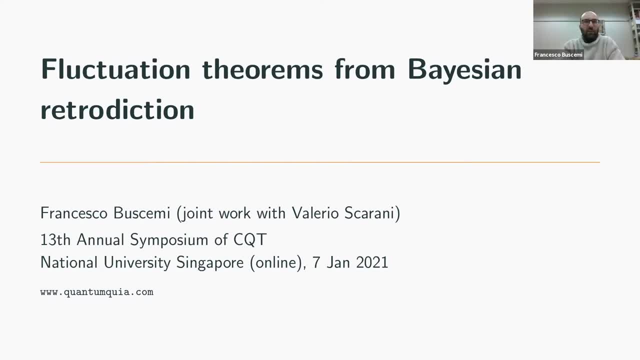 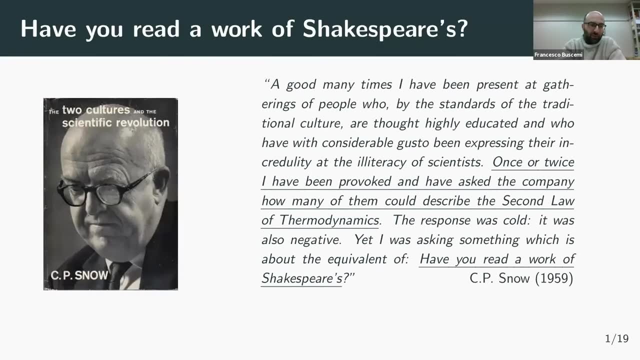 physics, And surely the second law enjoys a special role in physics And, like Shakespeare's, probably Shakespeare's work in English literature. So this is a quotation from a book by Charles Snow. So Charles Snow was a British scientist and novelist, And in 1959, he gave a lecture that then was published in this book, lamenting how science and the 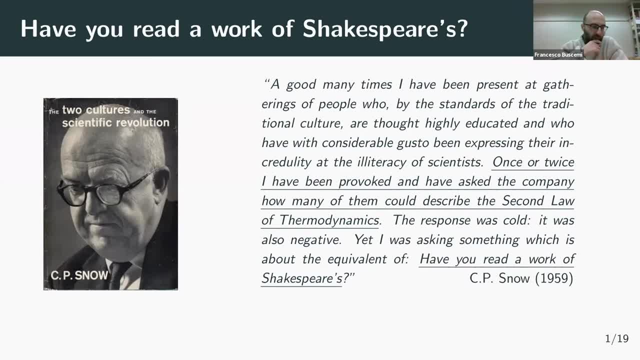 humanities, which had been closely intertwined for centuries in Western culture, have then split, have ultimately split into two blocks after disparaging each other, And he writes this. A good many times I have been present at gatherings of people who, by the standards of the traditional, 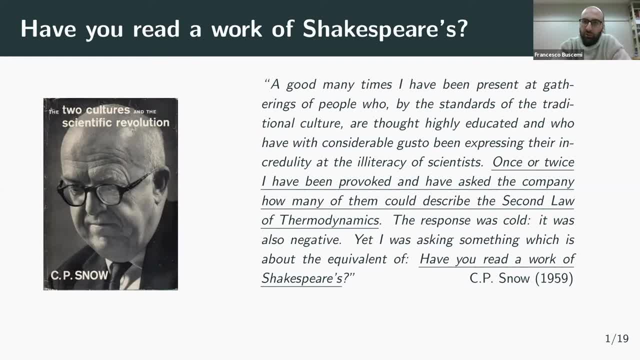 culture, are thought highly educated and who have, with considerable gusto, been expressing their incredulity at the illiteracy of scientists. One or twice I've been provoked and have asked them: Become illiterates of scientists by asked the company how many of them could describe the second law of thermodynamics. and the response: 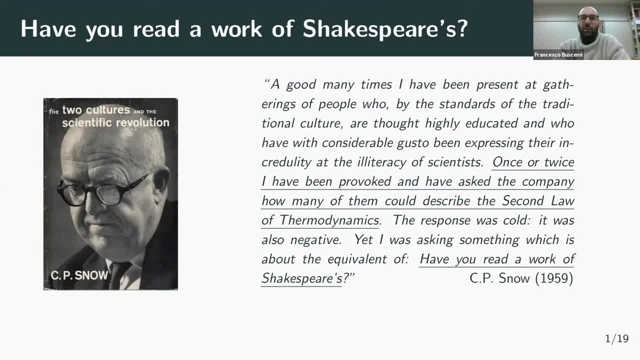 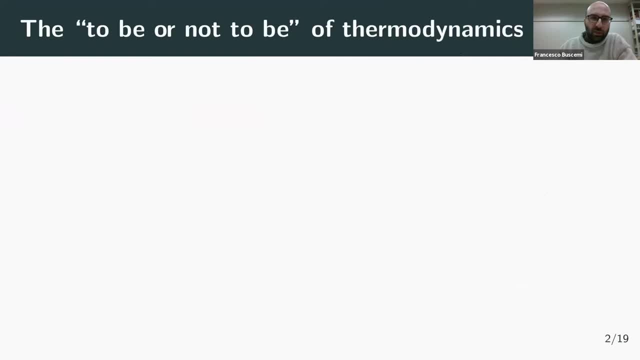 was cold, Yet I was asking something which is about the equivalent of: have you read a work of Shakespeare's? So what is the to be or not to be of thermodynamics? This is something that goes under the name of Claus's inequality, and it tells you- well you can say- that the entropy always increases. 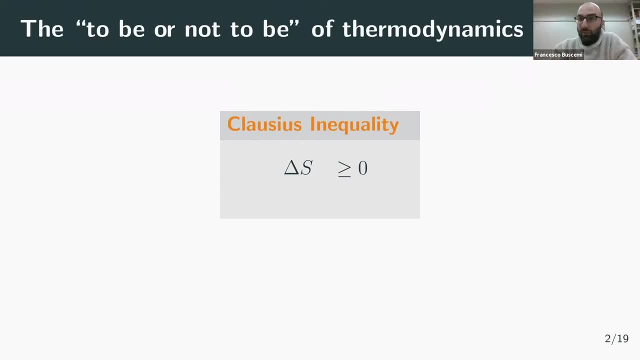 Or wait a second, like one can be more specific in this. This could be, like you know, the layman presentation of the second law, But then one could say, no, no, wait a second. that is not completely correct, because it is the entropy in the universe that is increasing, But since someone may, may. 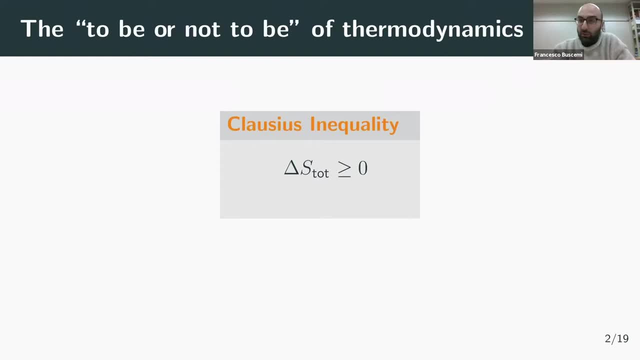 find issues with this formulation, because entropy is a statistical concept, so it's not that it is increases, but it's average the thing that increases. And then, actually, in your explanation of the second law, if you get caught by someone asking you, 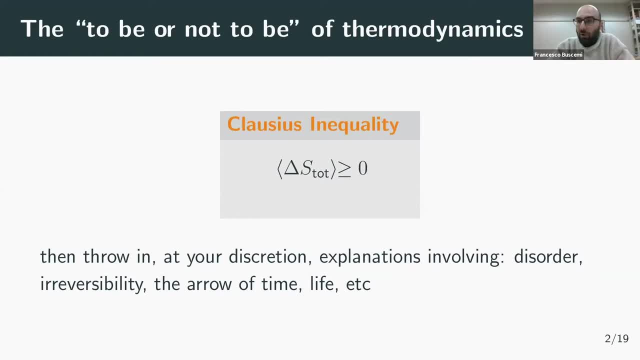 about the second law. in a fancy party, you can throw in at your discretion explanations involving disorder or irreversibility, or the error of time of life itself and so on In this sense, so all these things are extremely evocative and potentially deep. 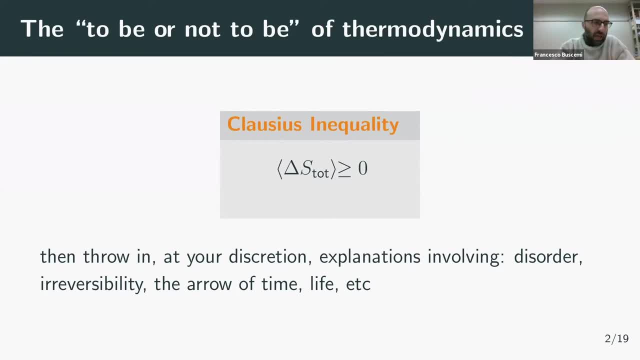 but not always, but do not really help a true understanding of the content of the second law, in my opinion. In this sense, I find that the second law from this viewpoint- only because it would be in a completely different ballpark- is similar to Gödel's incompleteness theorem, something. 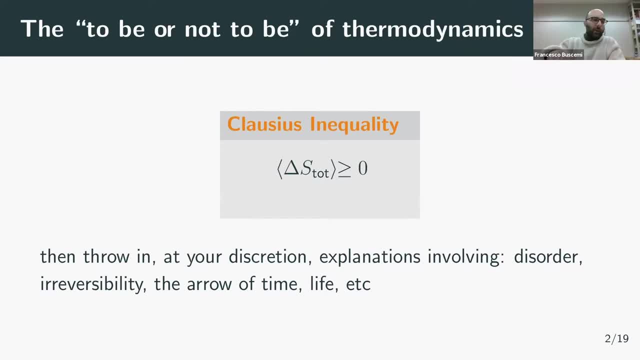 that is being popularized a lot, but often in the wrong way. But that is another story. So let's go back to Shakespeare. So, to be or not to be, how does it go on? That is the question. indeed, And as this guy, John von Neumann, 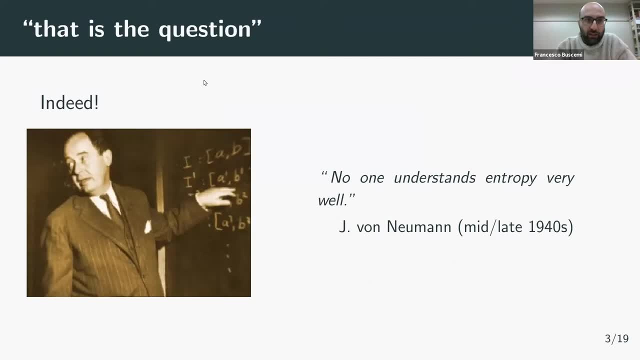 which is one of the smartest and brightest minds of the 20th century, said: no one understands entropy very well, And if John Neumann himself said that, you can trust me that entropy is quite a tricky concept. So let's try to formulate the second law without entropy. 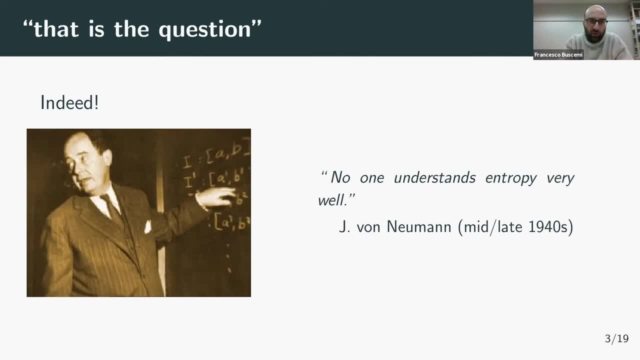 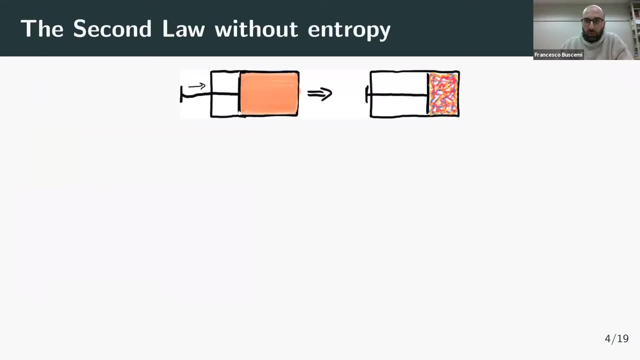 And that is possible. Actually, the second law need not necessarily involve entropy in its formulation, And it is as follows. So you can imagine that you have a piston with a gas inside and the gas is brought to thermal equilibrium with some surrounding environment. 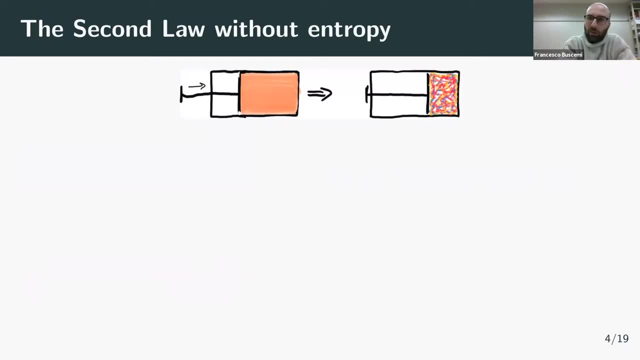 so that you start with an equilibrium state. Then you isolate the piston and you plunge the piston in, So you will be doing work on the system, And the second law in this case can be formulated as an inequality between the average work that you do by pushing the piston in. 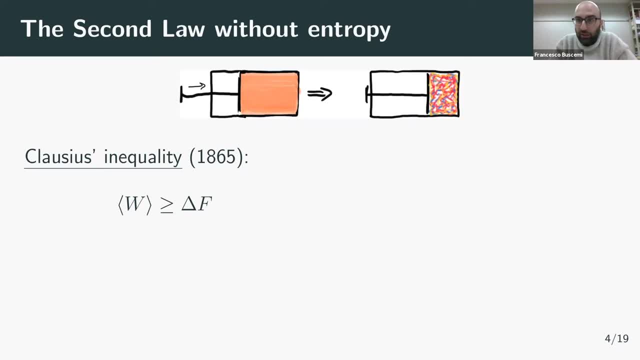 and the difference of free energy, which is somehow the energy that you can get back by letting the gas expand. You can think about it more clearly if you think about a cycle, So that you plunge the piston and then you bring the piston back to the initial position. 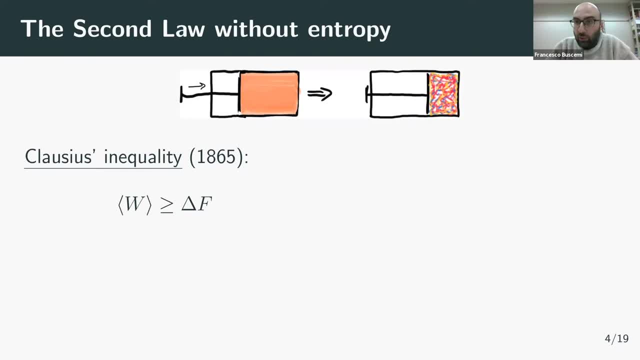 And this tells you the Clausius inequality tells you that if you are lucky, if you are smart, you are not going to do any work on the system, But typically you will have to do work. just to go back to the initial case. 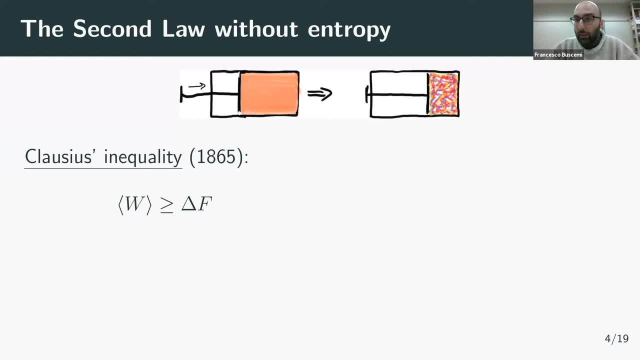 It's a kind of no free lunch result in building up thermal engines. So here there is no entropy, There are work and free energy, And this is one of the most important formulations of the second law. It is quite surprising to learn that. actually what? 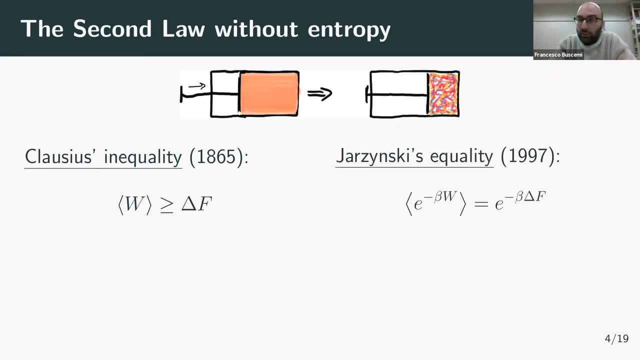 is an inequality can be actually formulated as an equality. This was done more than 100 years after Clausius' inequality was formulated by Christian Jinski in 1997, who actually noticed that by putting these terms in a different shape. so instead of having the average of work on the left-hand side, 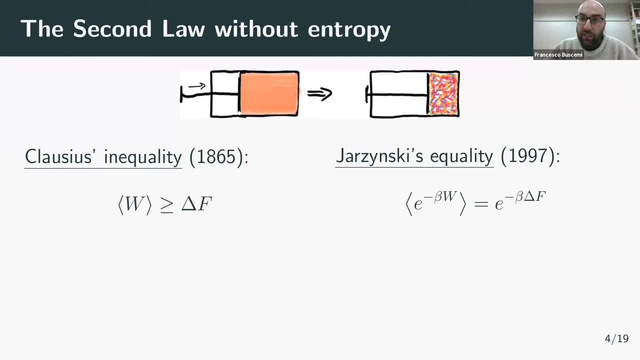 and the difference of free energy on the right-hand side. you take the average of the exponential of work now And this turns out to be equal, given some assumptions in the physical model. But for example, in the physical model I presented here, 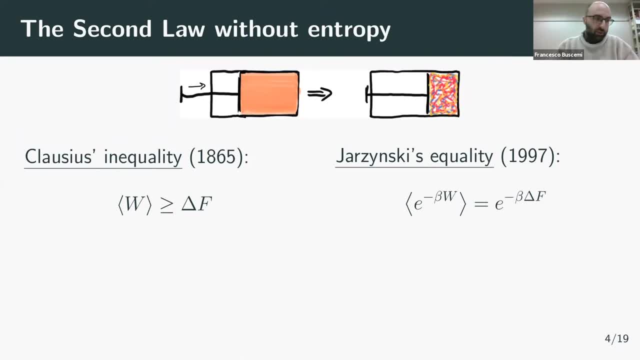 this is true, equal to the exponential of the free energy. So here you are looking at properties of the work distribution. So you have to imagine that work is something that can fluctuate. You can repeat the same process many times. 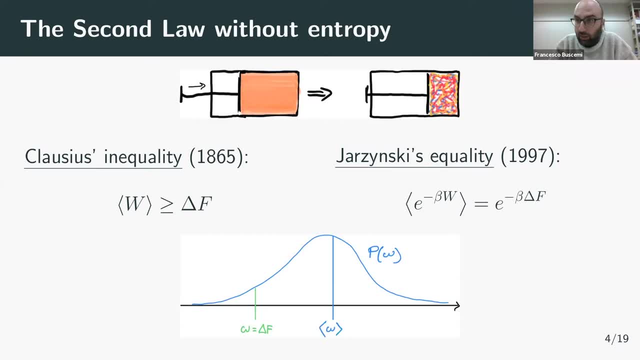 And every time you will find a different amount of work was needed or extracted from the system. This is something that we don't see naturally in our macroscopic world, And that is probably something that is probably also the reason why These jargiski equality was not discovered- until people had not 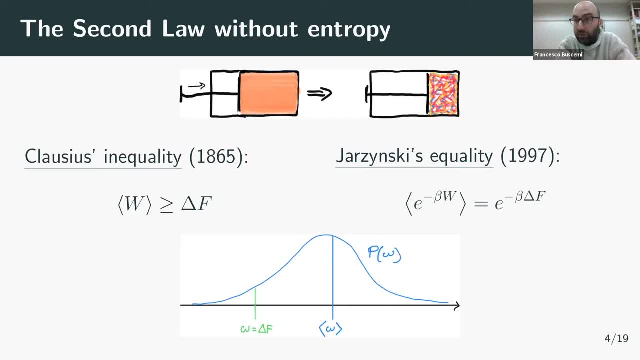 been looking into really small, The thermodynamics of very small systems, Because this parameter beta here is an astronomically large number: it is of the order of 10 to the 23. And so only extremely small fluctuations. surprisingly, here. In a sense you can say that this distribution of work for macroscopic systems 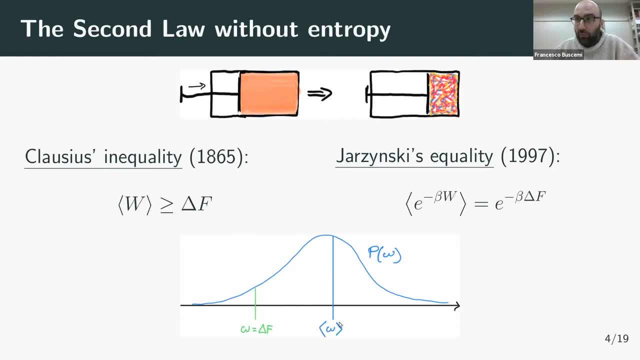 become extremely peak around the average value. So this is probably the reason why people have not been looking into this phenomenon before, but it is there and can be measured. If you measure work for small systems, you can actually see work fluctuating and you can see that fluctuations of 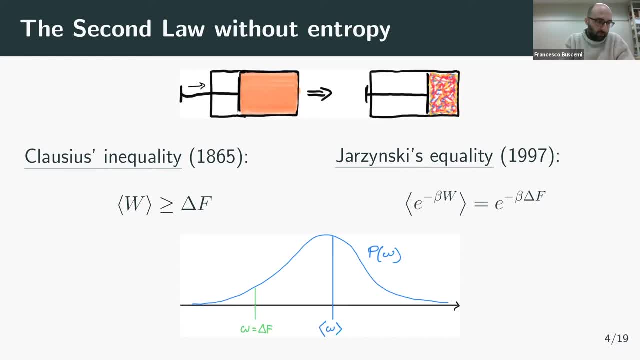 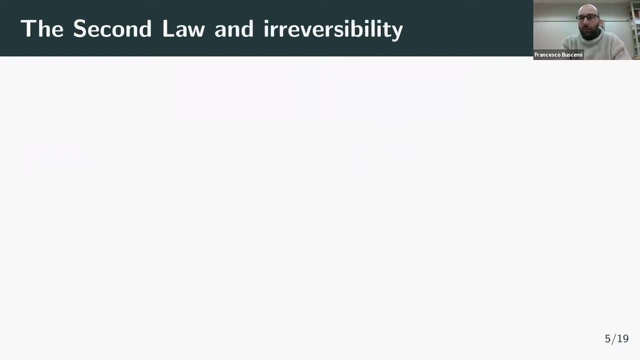 work obey Yerzhinsky equality. So now the problem is how to understand why this happens. So why is it so that Yerzhinsky equality holds? And in order to understand where Yerzhinsky equality comes from, it is helpful to consider not only the yin. 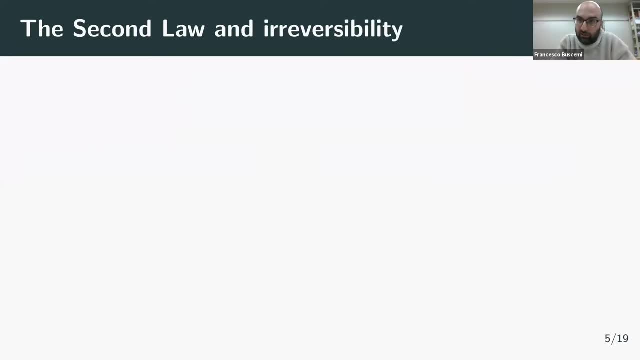 of this process, so, like the forward process, but also the yang, the version of the process, which is the reverse process. So, by continuing the simple thought experiment that I presented before, the forward process will be to plunge the piston in and the reverse process will be to start. 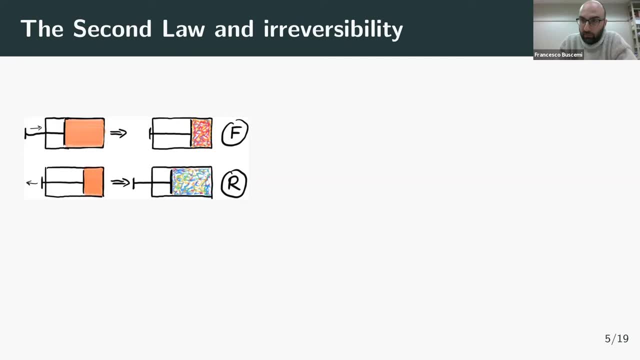 now, with the piston in the compressed position, with a system that is in equilibrium. Okay, so now it's equilibrium and it's compressed position, and extracting the piston out, This is the reverse process. So notice that while the initial state is at equilibrium, 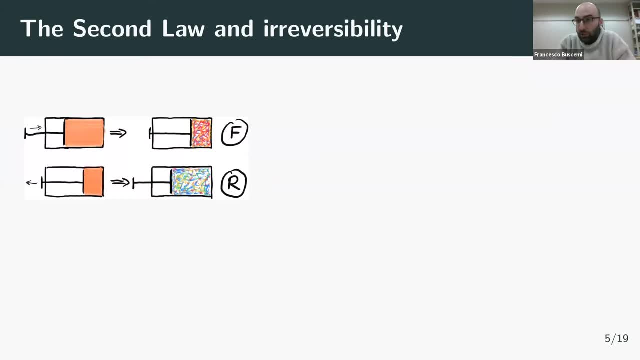 the final state need not be in equilibrium. So this is a very general thing. In a sense it is. it is an an easy experiment to implement. So and what do we know here? Hmm, Hmm, We know, We know fluctuation theorem. that was formulated just a couple of years after Yerzhinsky equality, in 1999.. 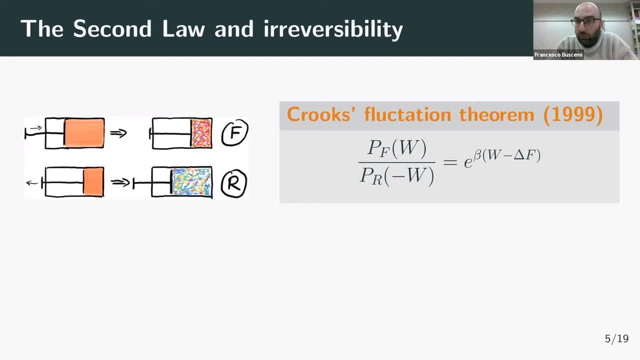 And this is a remarkable relation that relates the probability, So this is the probability density of work. So it relates the probability density of work in the forward process and the probability density of minus work, So the probability density of extracting work in the reverse process, pointwise, by means of this relation. So the ratio of these two numbers, 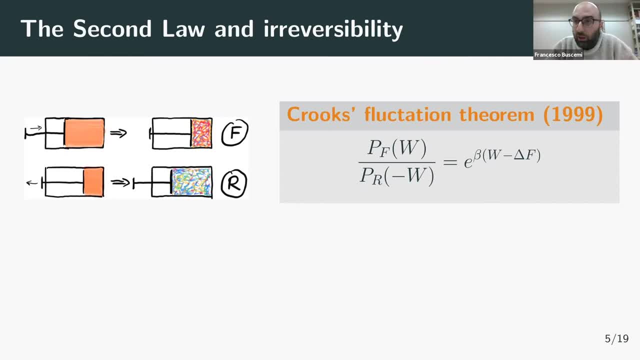 is equal to the exponential of work minus delta f, the difference in free end. So again, let me tell you again that this beta is huge: 10 to the 23.. And so these fluctuations are there, And you see that these two numbers are of a comparable order of magnitude. 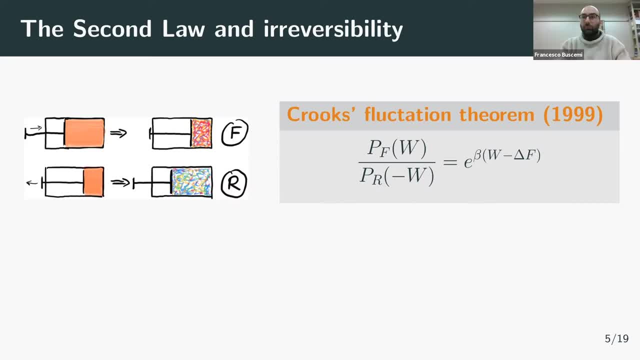 only when fluctuations are extremely small. Otherwise, for macroscopic differences, for macroscopic values of work, then these numbers is extremely in favor of the forward process. So you have a kind of a symmetry between the work distribution in the forward process and the backward process. 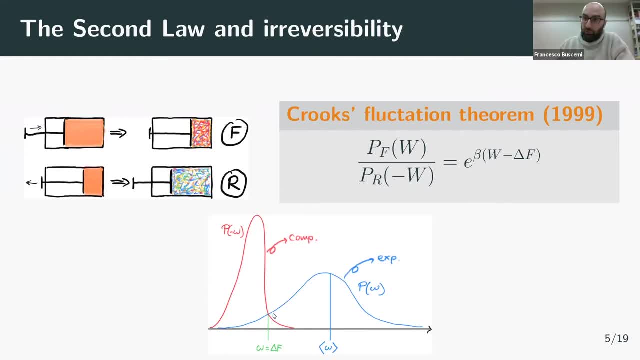 But the remarkable feature of these two things is that they cross exactly at the difference of free energy. So these curves can be whatever, They can be very far from the Gaussian and so on, but they will cross at the difference of free energy. By the way, maybe I should mention that these relations were 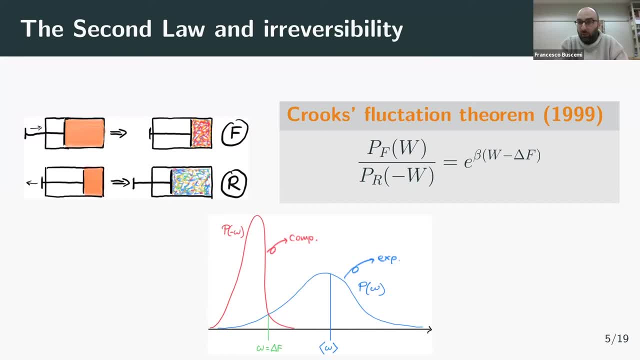 already presented in 1977 in a paper by Bochkov and Kuzovlev, but people say that they were doing something slightly different. But anyway, it is something that has been. you know, it is a field of research, research about fluctuation relations that exploded in the late 90s and we have to. 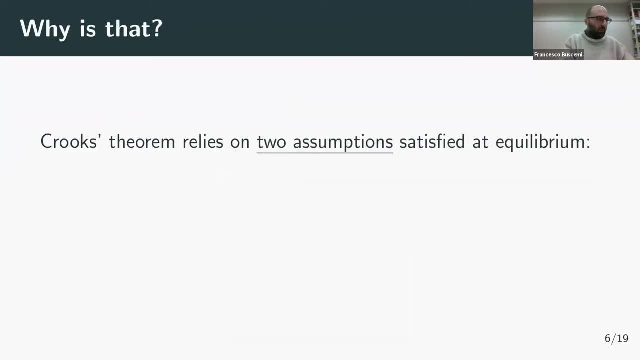 acknowledge that. Thank you, Thank you, Thank you. So I could go on and say so. why is that So? why Krupp's fluctuation theorem holds. So we started from the second law and we tried to make sense of it And we said: well, 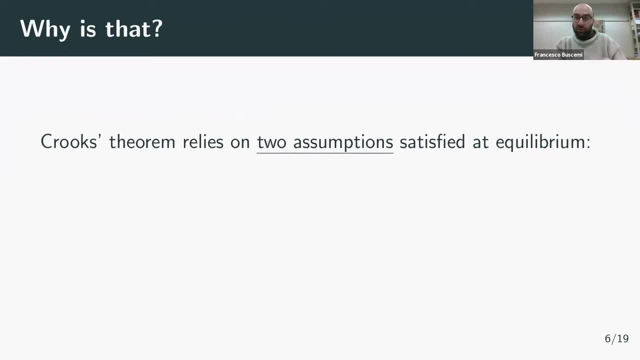 we went to a more general formulation of the second law, which is Yerzhinsky equality. From Yerzhinsky equality you can derive the second law just by using the convexity property dimension function. Now we have something, in a sense, that logically comes before Yerzhinsky equality, because 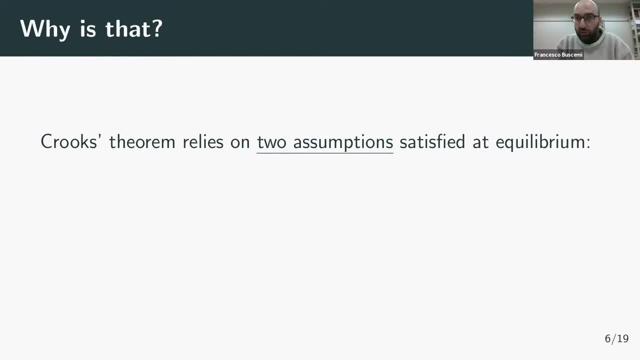 from Krupp's fluctuation theorem you can derive Yerzhinsky equality as a consequence. So now it would be interesting to see what are the assumptions on which Krupp's fluctuation theorem relies upon. And these are two assumptions that are satisfied with equilibrium. The first assumption is that 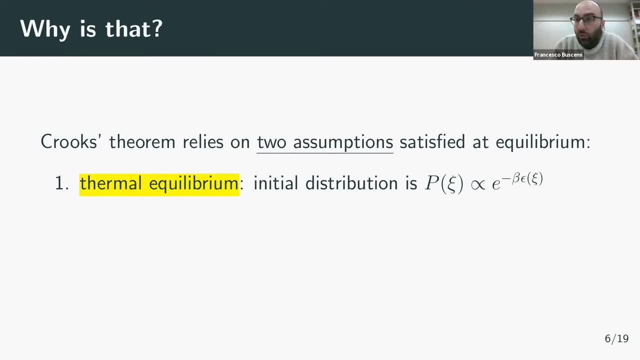 a system in thermal equilibrium is distributed according to the Ip's distribution, the thermal distribution And. the second assumption is that a system in thermal equilibrium is distributed according to the Ip's distribution, the thermal distribution And. the other assumption is that the processes that are going on inside the system. 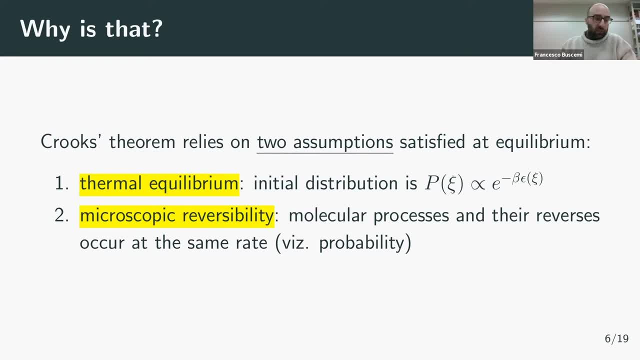 satisfy microscopic reversibility, which means that molecular processes and their reverses occur at the same rate, That is to say occur at the same probability. The probability of observing a trajectory forward in time is the same as the probability of a trajectory forward in time. 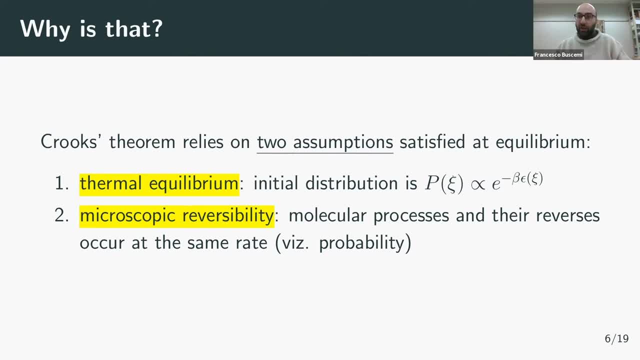 The other assumption is that time pulls down inside the system, so obviously there is no probability of observing the reverse trajectory when time is reversed. So it seems. so this is good, Good and well, everything is fine now. but it seems then that 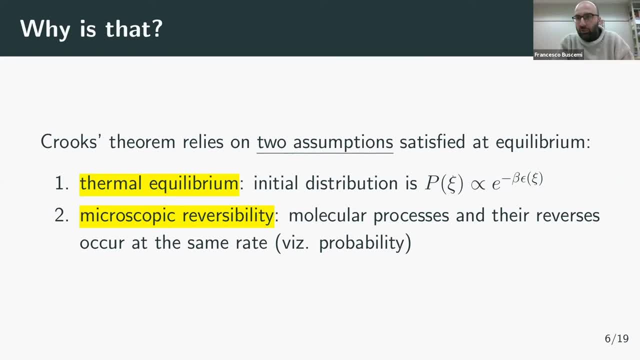 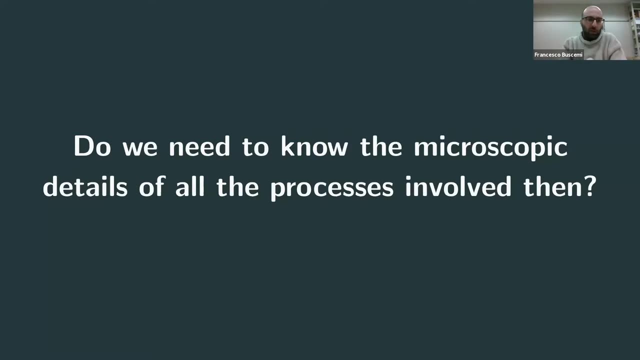 the second law, or at least Krupp's fluctuation theorem, which implies Yerzhinsky equality, which implies Clausius inequality, which is the second law, somehow depend on some microscopic balancing mechanisms that occur in the processes involved? So the question here is: 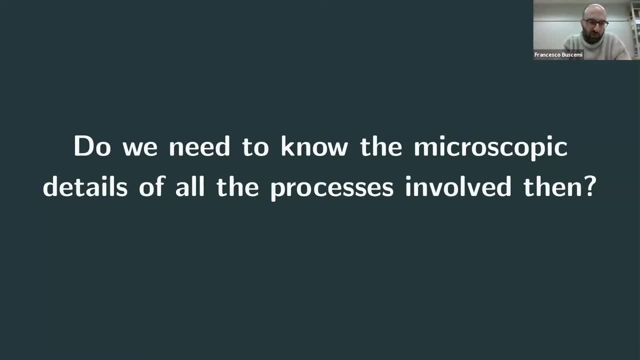 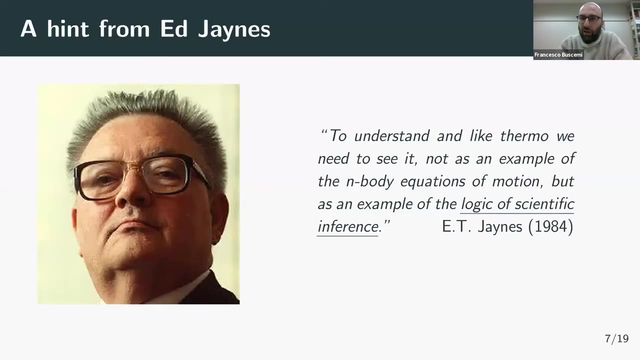 do we need to know the microscopic details of all the processes involved in order to say whether the second law holds or not? Is it some kind of universal property of microscopic interactions? This is something that I'm not so keen about, and I would rather follow the suggestions of Edwin James. 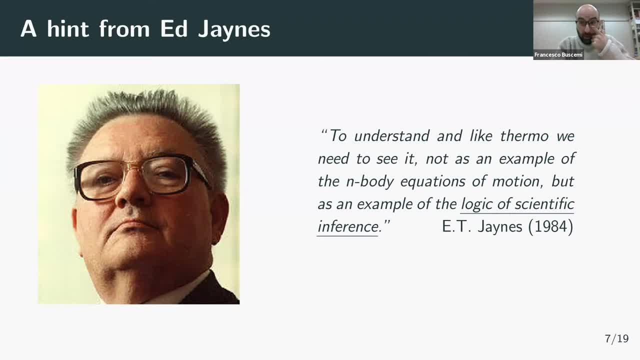 who writes in his paper the Predictive Power, Predictive Statistical Mechanics 1984, who understand and like thermodynamics. We need to see it not as an example of the n-body equations of motion, but as an example of the logic of scientific inference. 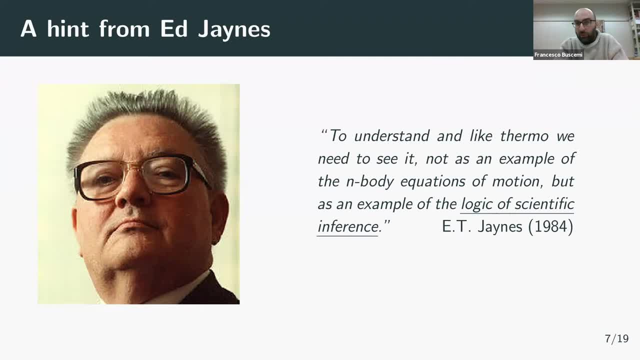 And the main idea in this talk is to basically follow this, So to try to see whether Crookes fluctuation theorems actually really rely on some assumption about the macroscopic processes that go on inside the box or whether it can be just derived by consistent logical thing. 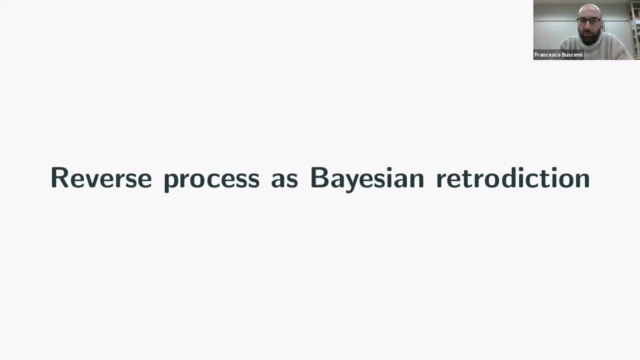 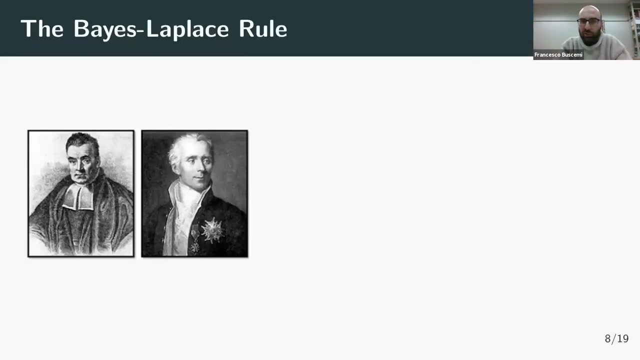 And here we come to the main part of my talk- a reverse process as Bayesian retradiction. So everything Bayesian starts from Bayesian Bayes rule, or to be more precise, the Bayes-Laplace rule. So Bayes Thomas Bayes wrote an essay. 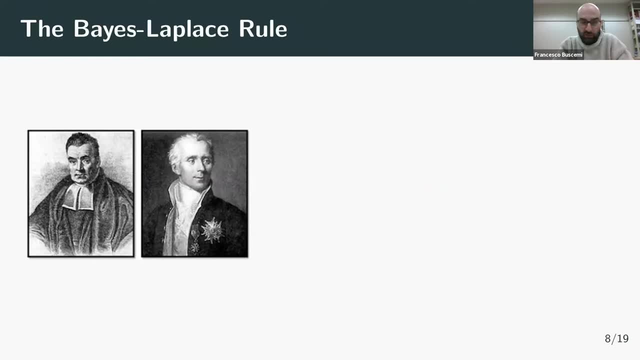 that was never published during his life was published after his death, where he proposed some method to consider the probabilities of hidden causes, which is what later has been generalized independently and formalized in the form that we know now by Piassimon-Laplace, who lived roughly 50 years after Bayes. 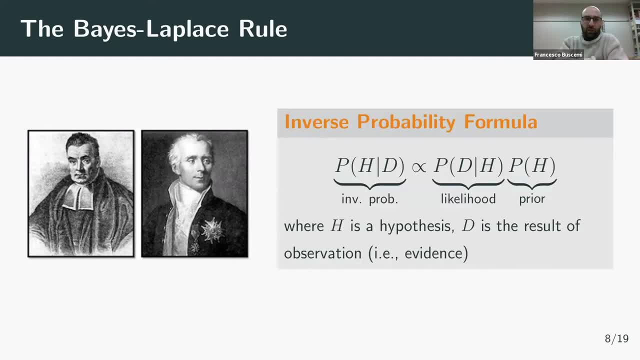 So the inverse probability formula, or the Bayes-Laplace formula, looks as follows. It is something that is in elementary textbooks, in probability theories, taught to first year undergraduates. So it tells you how to update a prior probability formula, how to update a prior distribution that you have. 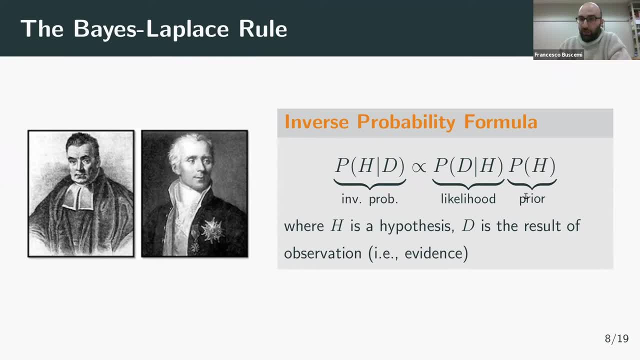 about a set of mutually exclusive hypotheses, P of H in the face of observations. So if you're given a data D, then you should update your knowledge, your information about the hypothesis behind the data according to this formula. So the answer to this last case. 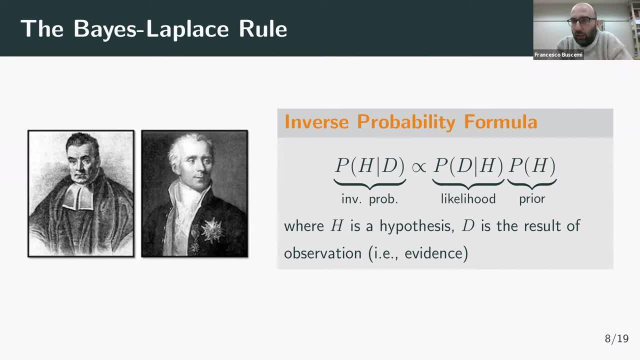 this is a delicious little person. I review my expectations of the table today. I have written hundreds of studies and, unfortunately, 11s and 14s of overall collection of these data in the past month, So I really don't want to get into the problem. 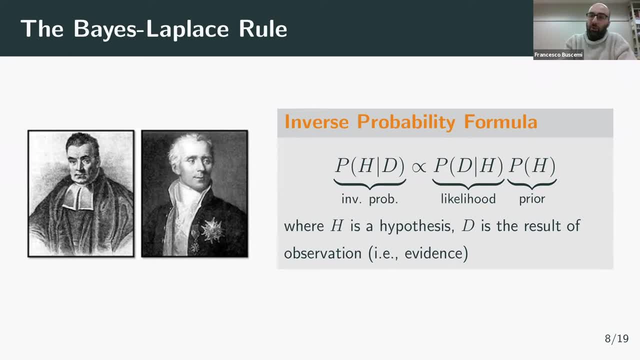 of the determination of the prior. this is a problem that has been beaten to death and we will be doing post-modern Bayesianism, so without necessarily subscribing to any particular ideology, but we will use Bayes' rule as a tool to do inference, statistical inference. 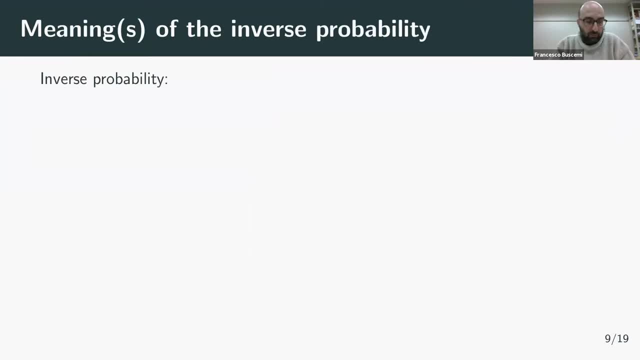 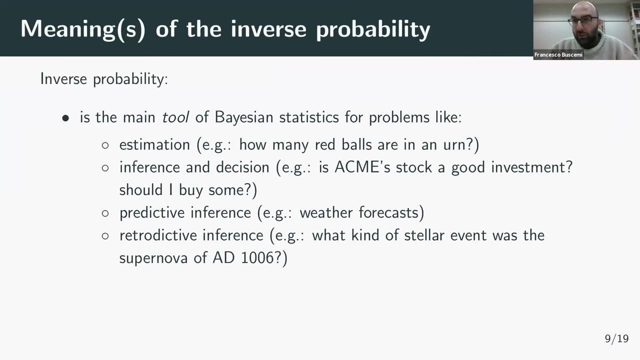 So what is the meaning of inverse probability? So inverse probability, as I said before, without putting too much interpretation on it, we can just see it as the main tool, as the main technical tool that Bayesian statistics uses to attack problems like estimation or inference and decision, and in particular predictive inference, particularly relevant in 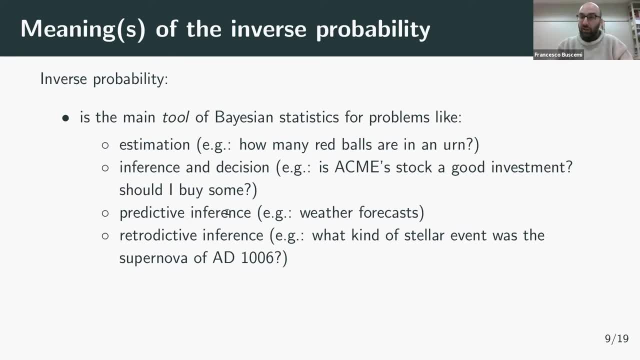 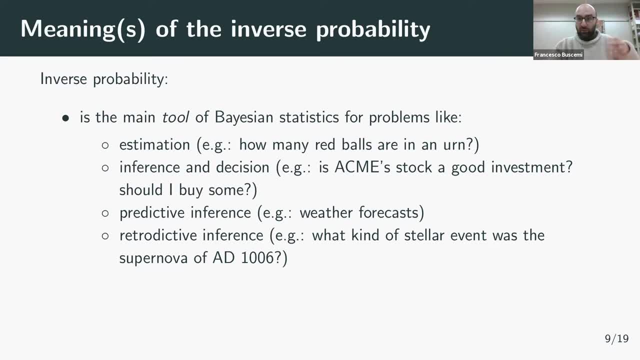 This is also the viewpoint preferred in physics. This was like the baseball picture of Ruth before, like that you start with some initial condition and then you bang, you let them evolve, but also with retrodictive inference, which is not any kind of magical things. This is something that is routinely done in 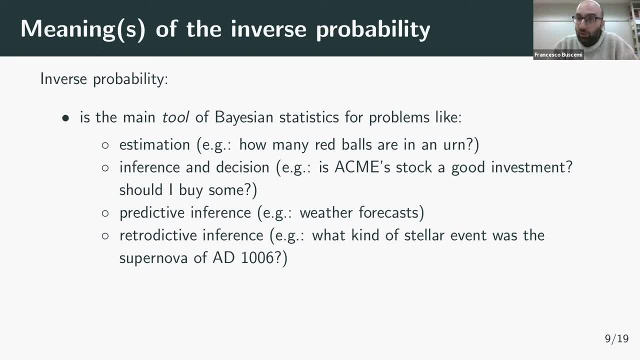 many branches of sciences, For example in astronomy, we can only do retrodictive inference. We cannot surely prepare some astronomical state and let it evolve right. We just observe passively data that come to us from the sky and we give them some scientific 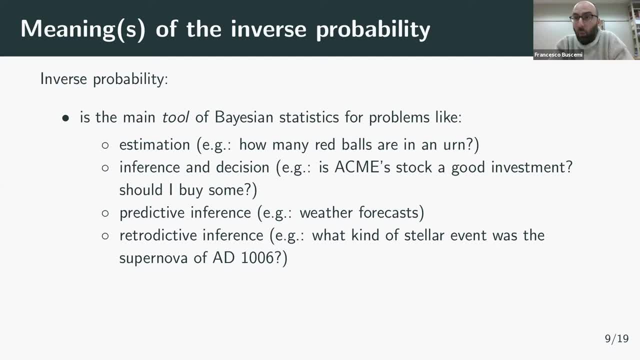 interpretation, You retrodict what these signals came from essentially. And inverse probability can be understood as the measure of the degree of belief in one hypothesis among other mutually exclusive ones, Given the data. So basically, Bayes rule, Bayes rule plus rule is the norm that tell us how to reason in a 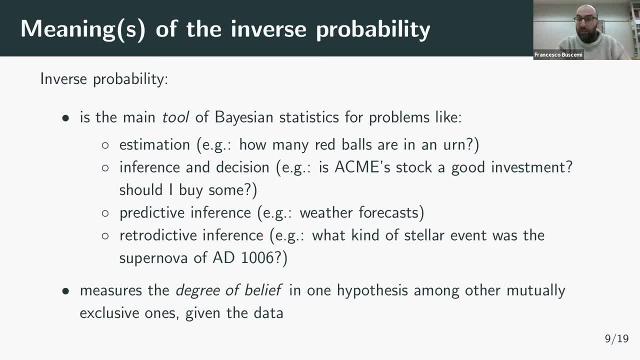 consistent way And it can be thought as a logic that generalizes Aristotelian logic. Bayes rule contains all Aristotelian syllogisms and has more. Actually, Bayes rule is closer to our natural way of inferring properties of the world. 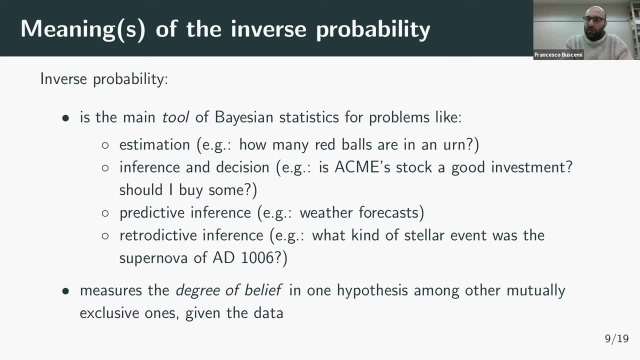 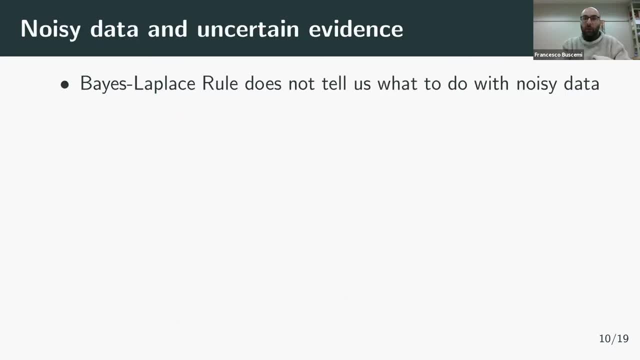 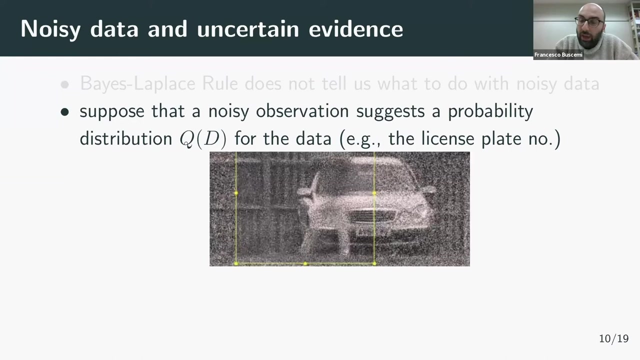 around us. There is a limitation, however, to the usage of Bayes rule as it is given in textbook. That limitation is the fact that Bayes Laplace rule does not tell us what to do with noisy data. So suppose, for example, that we have a noisy observation, which is actually what happens all. 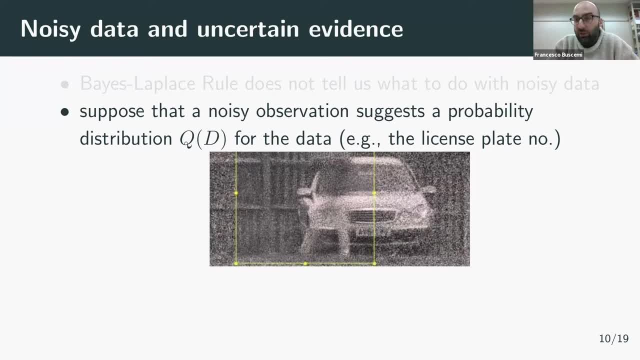 the times We never have noiseless observations. There is always some noise in our observations, more or less, but sometimes the noise is so strong that we cannot actually say that we got some data exactly. For example, imagine that our data from the picture we want to extract the data we would. 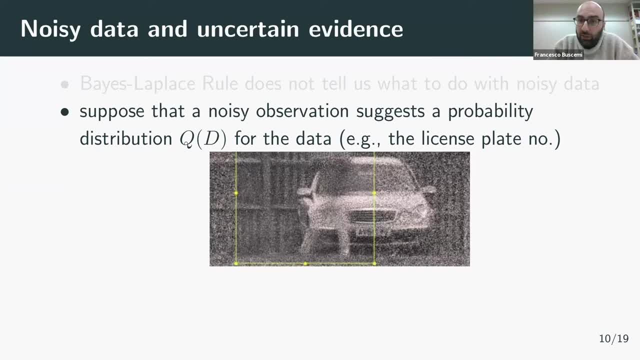 like to extract is the license plate number right. This picture is so noisy that we cannot say that we had. we can read any definite number on the license place of the car, license plate of the car. But we can give some kind of distribution, some kind of belief about what's written on on the 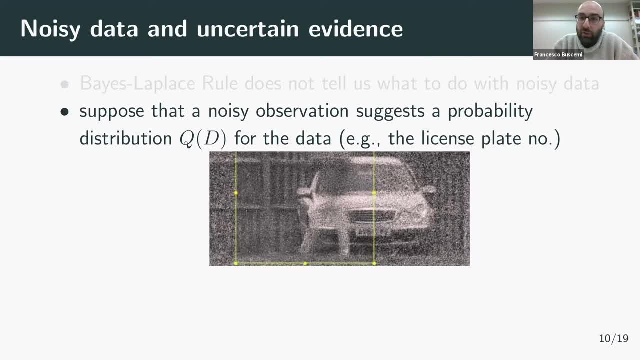 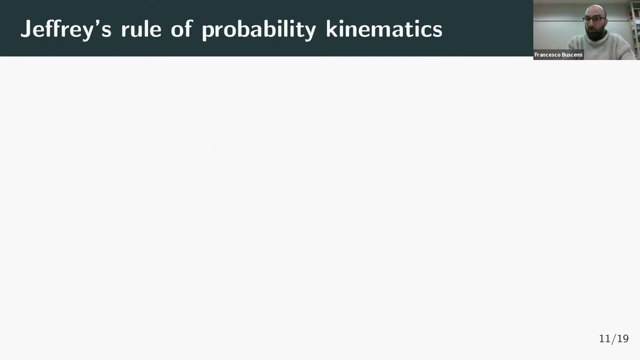 license plate of the car. So say that you have a noisy observation that suggests you a probability distribution to the on the data. should we update then our prior on the hypothesis given uncertain evidence? This is something that the Bayes' rule doesn't tell you straight away. So we need some new cookbook, some new rule to 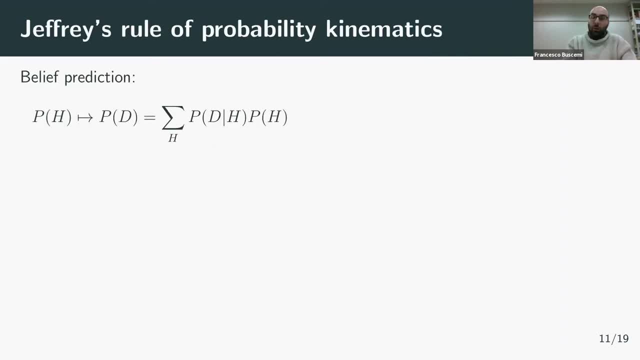 deal with noise observation, which constitute Bayesian retrodiction, exactly. So on one side, let me repeat, we have belief prediction which, starting from some knowledge about the hypothesis, propagate this knowledge through some process that can be seen as the process that generates. 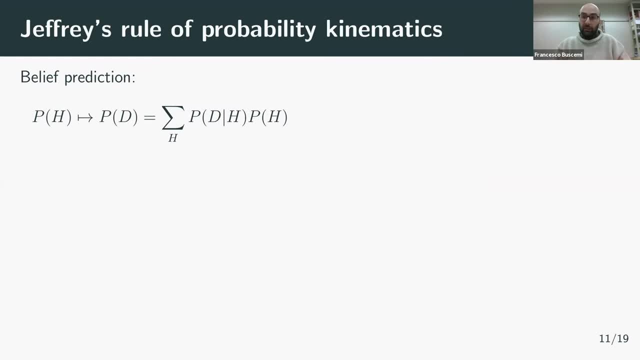 the data and we have the probability on the data. We can predict the distribution on the data. So how can we work instead with belief retrodiction? Say that we start with the belief assignment on the data. How can we back, propagate this belief on the? 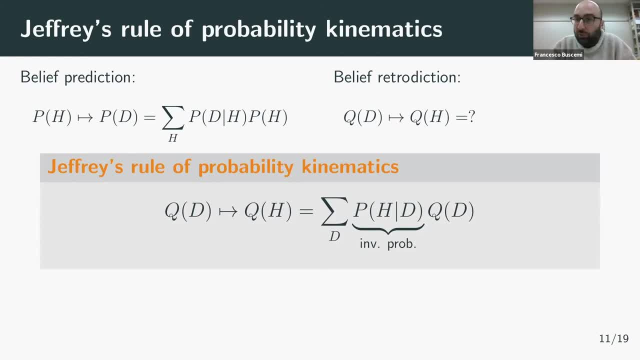 hypothesis. So we need Jeffery's rule, so-called Jeffery's rule of probability kinematics. This essentially tells you that if you have a noisy observation described in terms of a distribution over data, this should be back propagated on the hypothesis by means of the 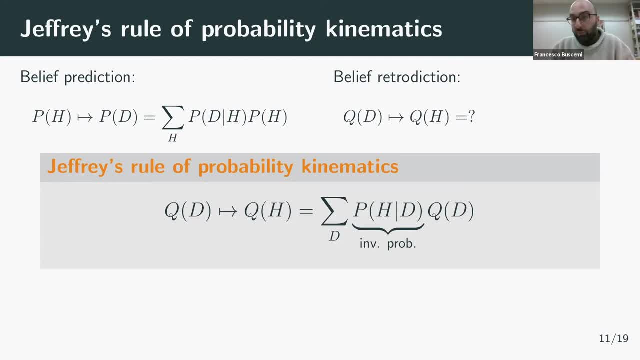 inverse probability that now is not just a number but becomes a process in itself. You see, it's a kind of noisy channel, applied on the probability distribution, on the data, To get the probability distribution of the hypothesis. So Jeffery's rule, which was introduced as a kind of an 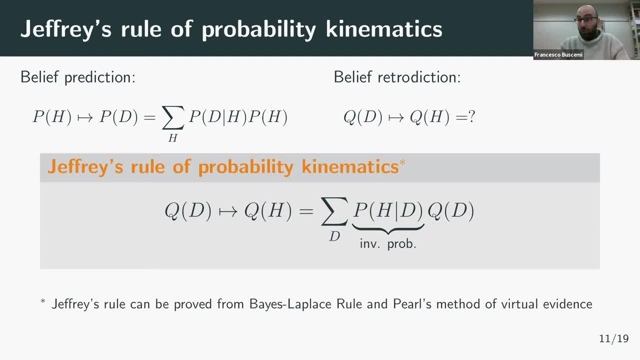 ad hoc theory in statistical inference can actually be proved from standard Bayes-Laplace rule and Pearl's method of so-called virtual evidence, but I won't go into that detail. Anyway, it is something that follows as a mathematical consequence from the usual Bayes-Laplace rule. 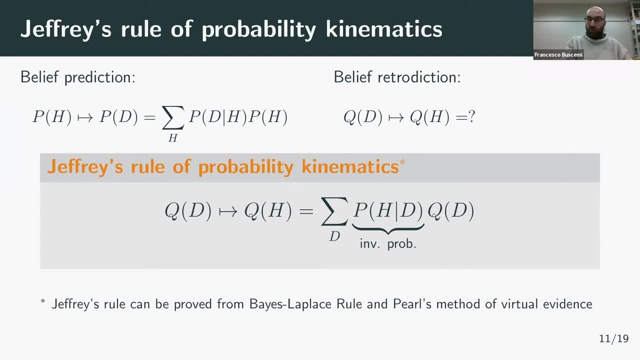 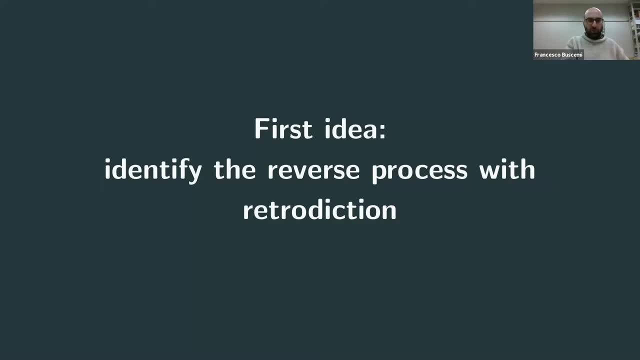 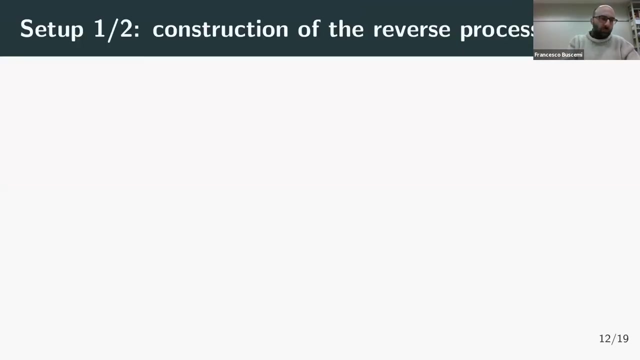 Okay, so Jeffery's process is what we consider as the retrodiction, as the reverse process. So the first idea here is to identify the reverse process when you're dealing with a stochastic process in statistical mechanics, with retrodiction. So how do we construct our setup? So we start from some. 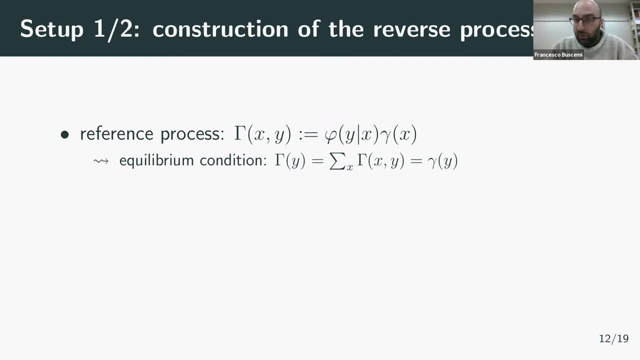 stochastic process. Here you have the initial conditions, the initial distribution of the states of your system, and here you have a stochastic process that tells you how this new state variable y, is distributed given the initial conditions. And you start from equilibrium condition typically, because usually fluctuation. 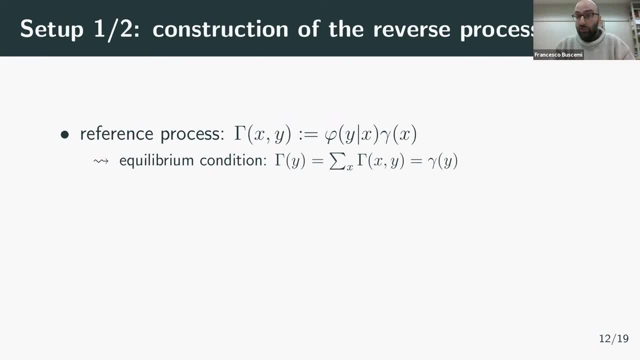 we are aiming at constructing fluctuation relations, and fluctuation relations are usually considered fluctuations around equilibrium. So you start from the equilibrium condition, so you search for a fixed point gamma of this stochastic matrix, and then you do Bayesian inversion. You just construct the inverse probability, but now the inverse probability. 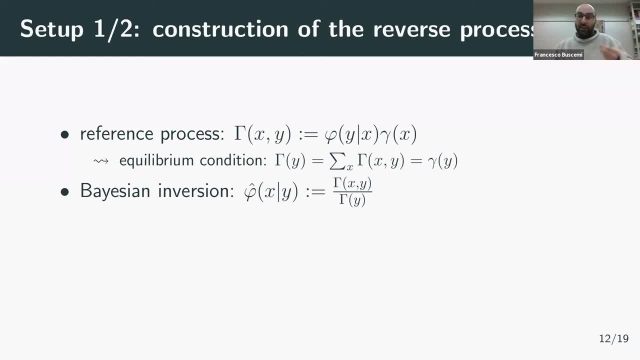 here is not just a number, is not just the updated prior, but is considered as a process itself, A process where the, if you plug into some knowledge about the state of the system at later time, it will tell you the thing that you should infer, the distribution that you should infer. 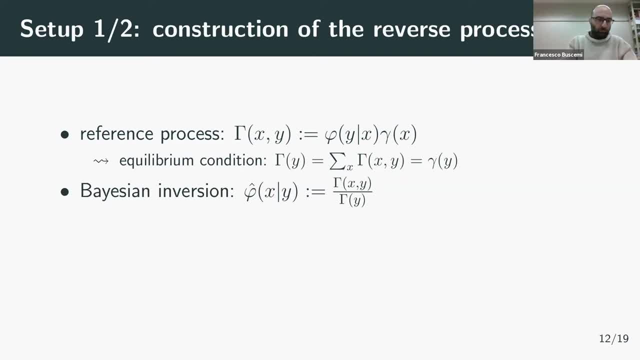 about the state distribution of the system at previous time And because we used a proper distribution, gamma equilibrium. this relation between reverse process or retrodiction, with the predictive channel, with the predictive process, the forward process, phi, is just given by this proportionality factor, which is a ratio. 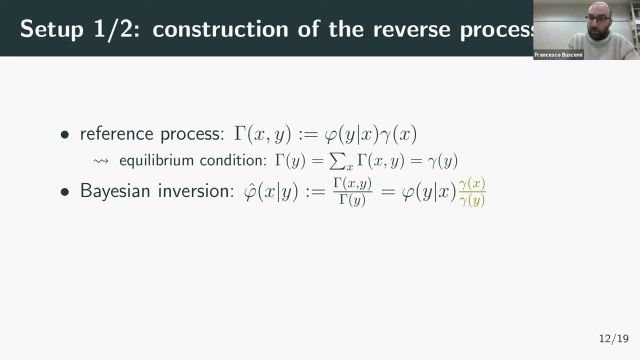 of the entries of the equilibrium distribution, the steady state. So at equilibrium, because we chose to invert, to construct the inverse process at equilibrium. at equilibrium, nothing happened. So prediction is equal to retrodiction. If we are observing a glass of water, for example, at room temperature, at equilibrium, nothing really happens. I can just. 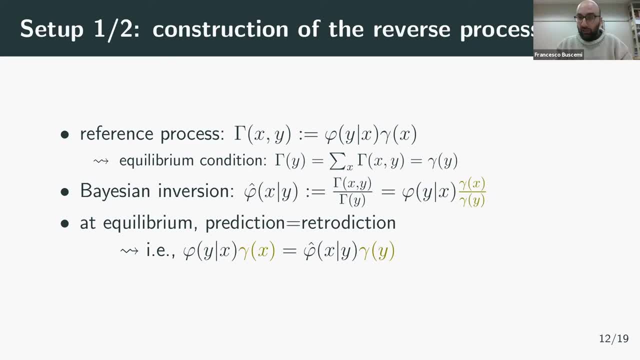 prepare it and predict what it will look like at later times. but I can just look at it now and predict and retrodict how it looked like before. It is already at equilibrium, so there is nothing to predict nor retrodict. It is there, It is something stable in time. It does not evolve, so nothing. 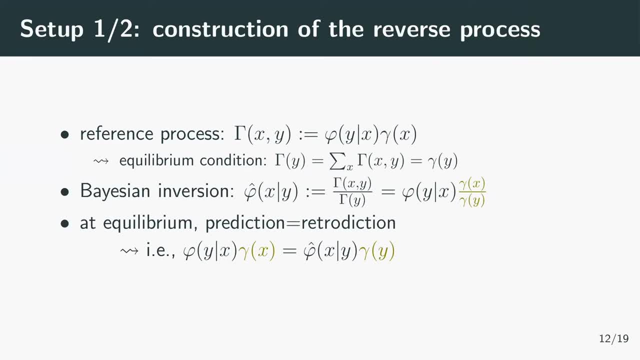 really happens. By the way, retrodiction in Hamiltonian dynamics it is just retracing trajectories in phase space backwards. So it is the usual idea, retrodiction. Sometimes also people. when speaking about the second law they speak about the reverse movie. You take a movie and you show it in reverse. 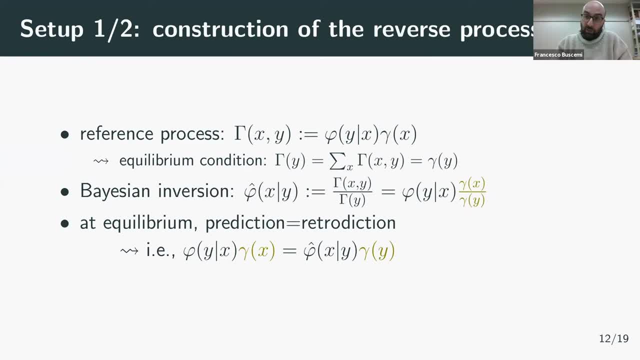 It is good, but we have to take these examples with a grain of salt always. But in Hamiltonian mechanics it is really true. If I reverse the movie of a planet going around the sun, you will not see anything strange going on. 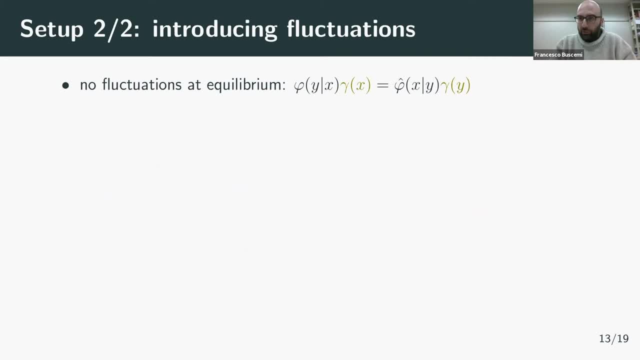 So the next step is to introduce fluctuations. So, as I said before, at equilibrium nothing happens. There are no fluctuations at equilibrium. But now we change our beliefs. So we imagine to be on one side, we imagine to be a predictor. 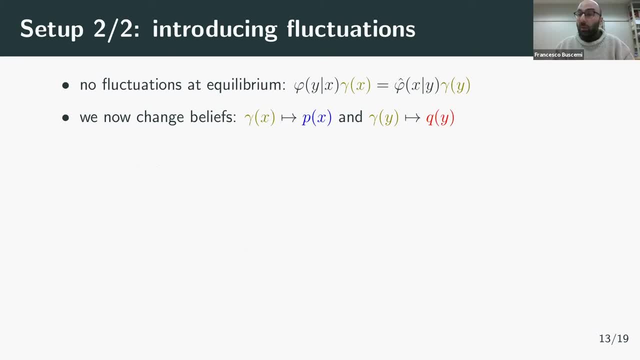 that changes the initial distribution to some other distribution- p of x. But on the other side we consider the situation from the viewpoint of a retrodictor that changes for some reasons, for example, in the face of some data Changes, updates this equilibrium distribution to another one and this is not in equilibrium anymore. 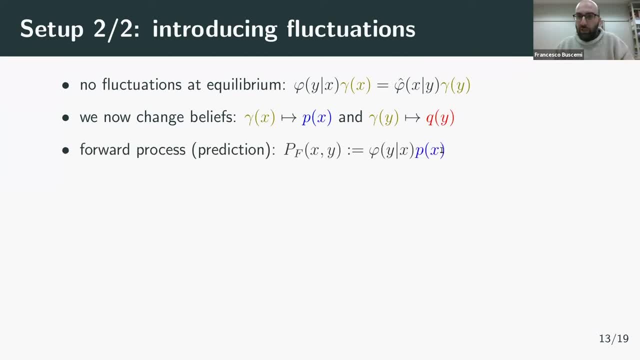 You can construct now a forward process, which is the evolution of this new prior is this new initial conditions, px. but you can also construct a reverse process using retrodiction, which is taking this new conditions of the final state and retrodict using those, uh, the probability distribution at prior times. so now we are out of equilibrium and so the 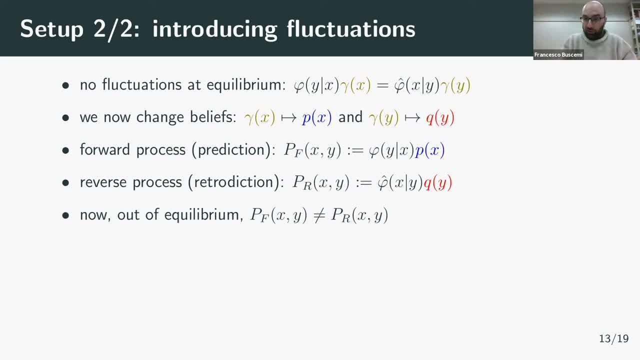 forward process is different from re, from the reverse process. you can see as a little cartoon as this. so at equilibrium you have the predictor and the retrodictor will essentially be doing the same job, but out of equilibrium. so if we replace gamma with different distributions, then the predictor is going to say something different from what the retrodictor will say. 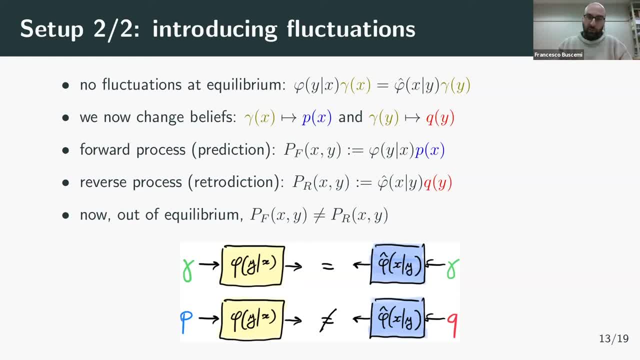 so, in a sense out of equilibrium, this symmetry, this inferential symmetry, is broken. i'm not speaking here about physics, you see that. i'm just speaking about a like the logical asymmetry that exists between prediction and retrodiction. there are no hamiltonians here, in a sense no microscopic reversibility. 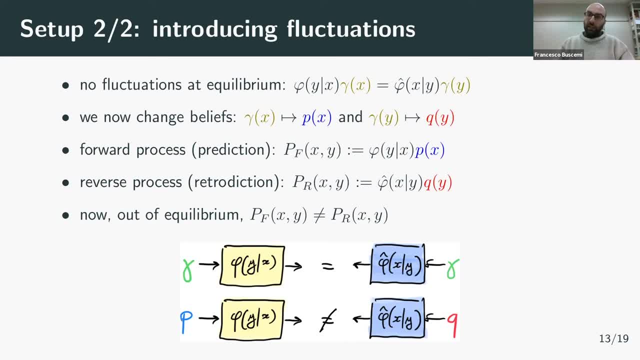 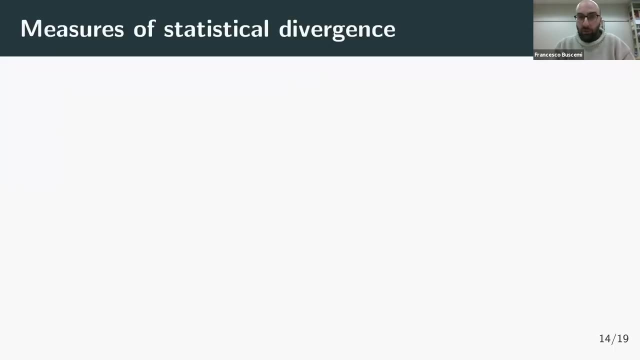 however, there is an asymmetry. so now the idea is that we want to quantitatively measure this asymmetry between predictor and a retrodictor using the tools of mathematical statistics. So we want to use some kind of divergence, So mathematical statistics. there are two big families of statistical divergences. 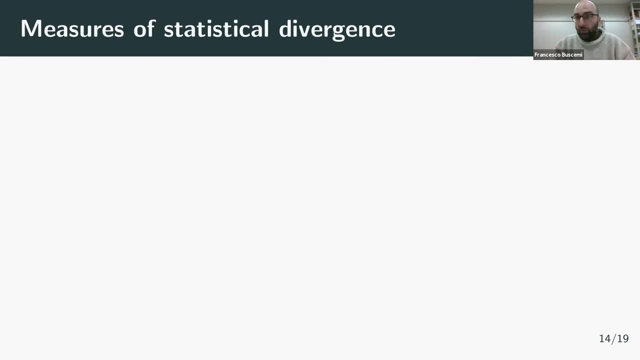 You have either F divergences that are being introduced later on or Bregman divergences that instead have a more kind of flavor like convex, analytical flavor To them. they are defined using Legendre, transform and so on. But F divergences, they start from the ratio. 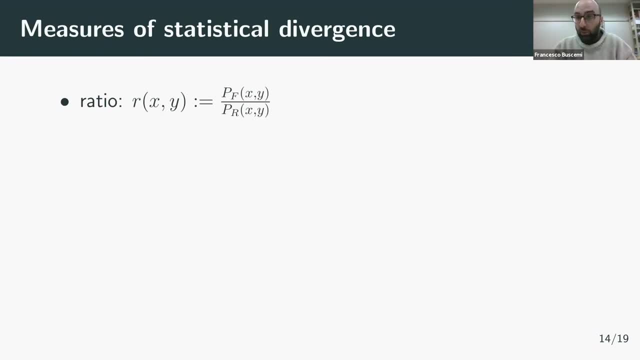 So you want to say how different PF, the forward process distribution, is with respect to the reverse process distribution, PR. So you construct the ratio, And here I'm not going to be worried about problems of zeros and so on, For the sake of this talk we only 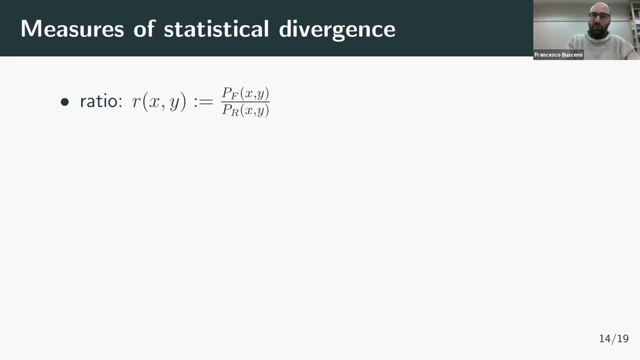 look at situations where these objects are always non-zero. So we define the ratio, which looks as this- I'm just replacing the definition of forward process and reverse process here And then, because we constructed the phi hat, the reverse process started from equilibrium. 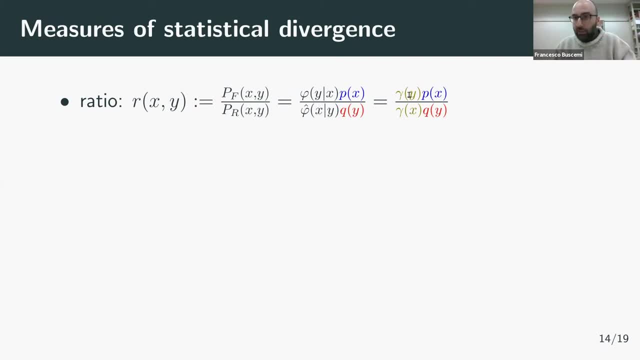 we can replace the ratio of the conditional probabilities by the ratio of the distribution and equilibrium. So this will be our starting point And then using the ratio, why we construct the ratio? We construct the ratio exactly because F divergences are defined as averages of this ratio. 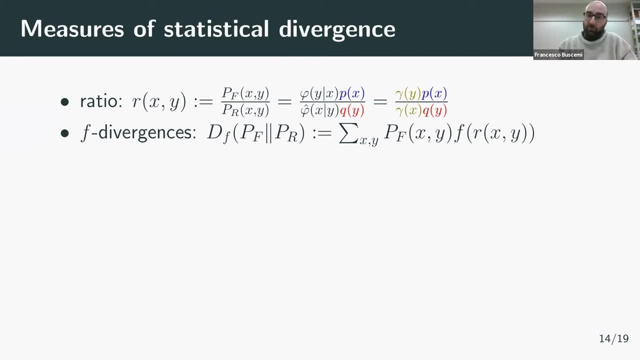 or better as averages of functions of this ratio. So an F divergence like this one is defined by giving a function F that has to satisfy some regularity conditions to be manageable, And then you take the function of the ratio and you take the average of this value. 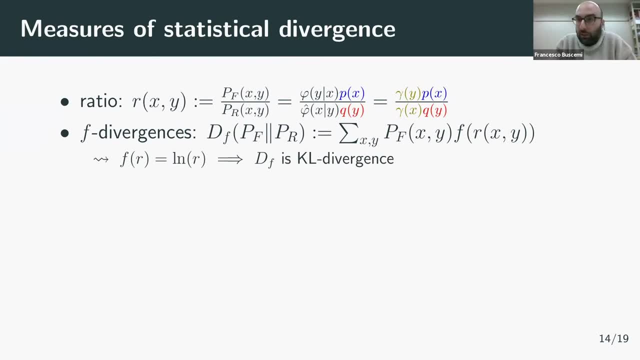 For example, if you take the function to be the natural logarithm, this function is exactly the Kullback-Leibler divergence, or the relative entropy, something that is extremely important in thermodynamics. quantum informant everything, But not only. 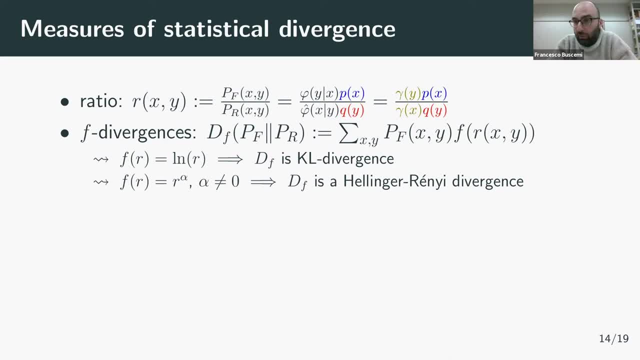 Because if you take this function to be some power alpha of R, then you have another very important family of statistical divergences, which are the so-called Hellinger-Renyi divergences. So here, for the sake of this talk, we assume F to be the Kullback-Leibler divergence. So here, for the sake of this talk, we assume F to be the Kullback-Renyi divergence. We assume F to be the Kullback-Renyi divergence. 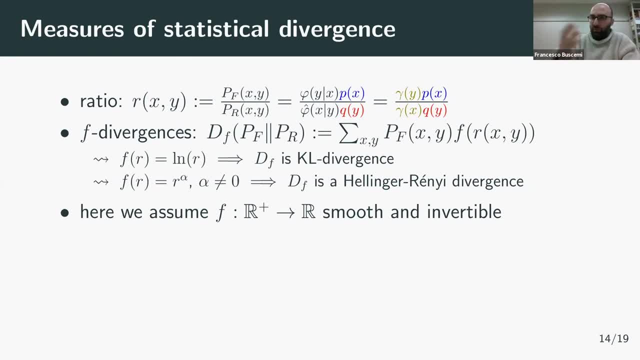 So here, for the sake of this talk, we assume F to be the Kullback-Renyi divergence, And then you take the function from positive numbers to R, that it is moved and inverted, For example, the logarithm will do. 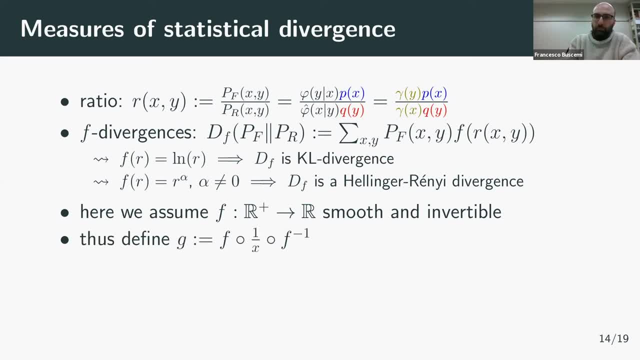 but also this R to the power of alpha, will do. And then we define some function, g, which is a kind of involution of f, by using the 1 over x, the inverse. Why the inverse comes up? The inverse comes up because if you want to exchange, 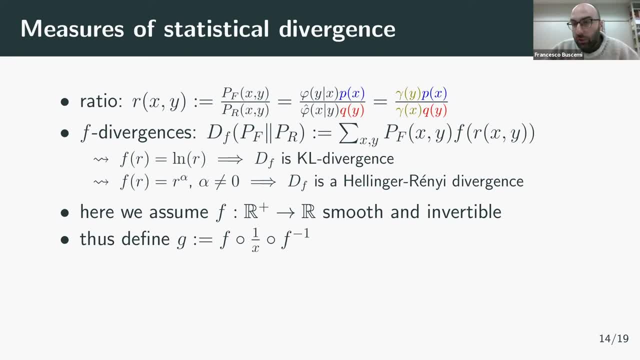 the role. when you exchange the roles of predictor and retrodictor, what does it happen? It happens that, but let us look at this ratio here. It happens that the new final condition and the new initial condition get, of course, an exchange role. What was initial before becomes final. 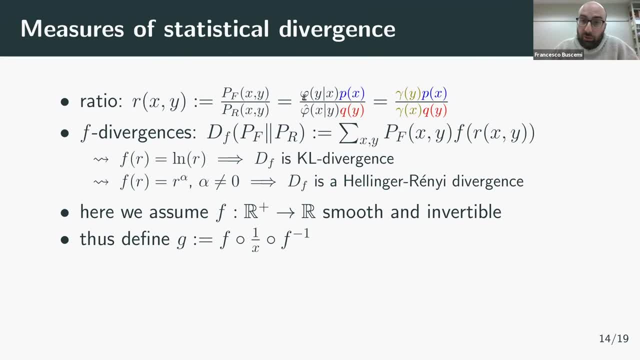 condition from the eyes of the retrodictor, but also the two channels, the two processes. change is role. So what is the forward for the predictor is the reverse for the retrodictor, and vice-versa. So that is why you have this. 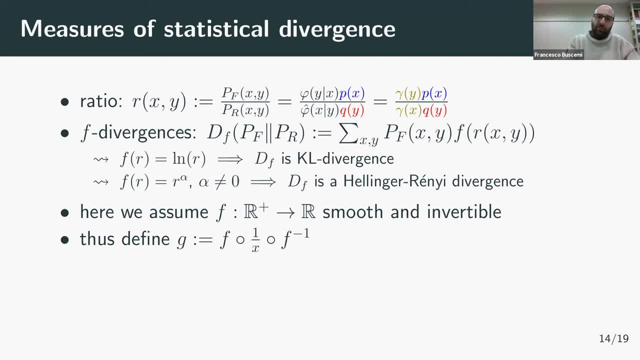 multiplicative inverse function in the middle. This is how you define this function. g, For example, in the case of the logarithm, g will be just minus r, Why? Because the inverse function is exponential. You have negative exponential. And this is only because the factor is just. 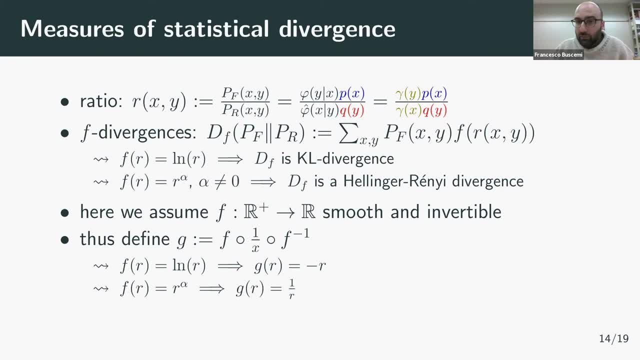 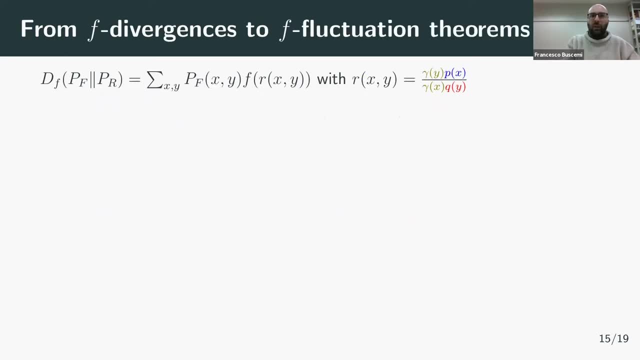 but just because our suppose that is doing the increasing of the operating current, if you take the logarithm of negative exponential you'll get minus x. In the same way, the g corresponding to the power law will be 1 over r. So now from f divergences to f fluctuation. 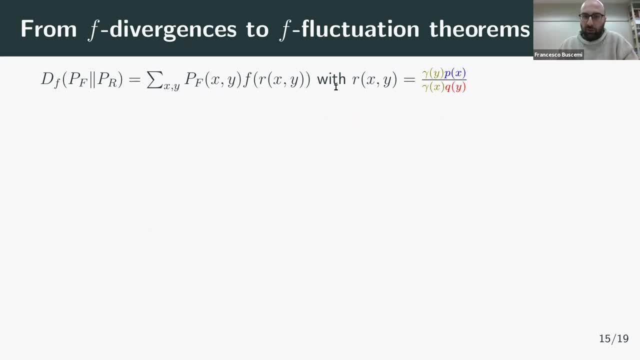 theorems. So we start from here again. I just reported the definition of f, divergence and the ratio, So now we want to. we are aiming at formulating fluctuation relations that are formulated usually in terms of a probability density function. So we introduce the probability. 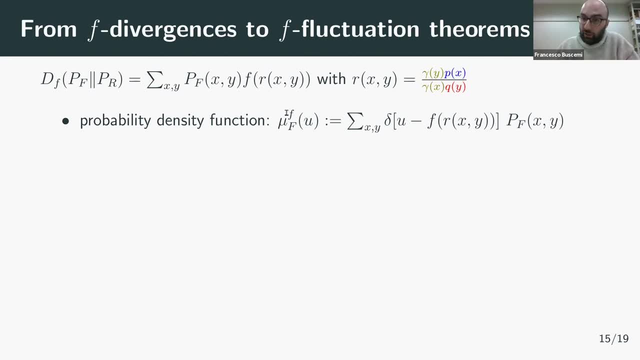 density function of this variable u for a given function in this way. So when the process follows this trajectory from x to y, we assign the value f of r to this parameter u, Otherwise you have just zero. This is a density function with deltas in this: discrete for discrete states. 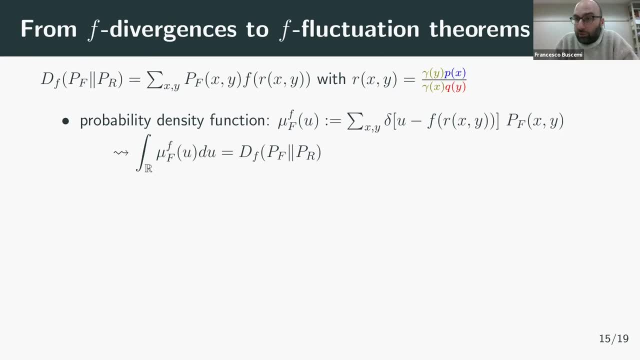 basically, But still you can. it is a distribution, So you can take now integrals And by definition, the integral of these things is exactly the f divergence between the forward distribution and the retrodicted, the reverse process distribution. So it is a measure of asymmetry. 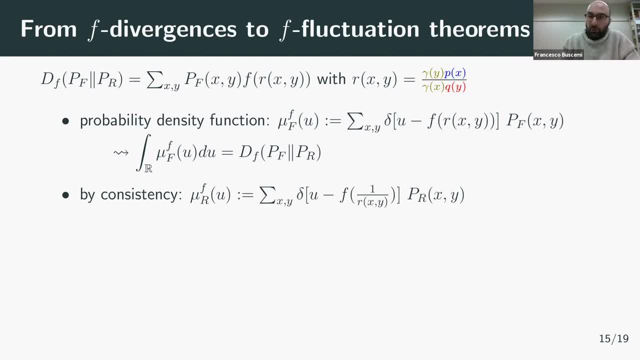 Now, by consistency, we want to introduce a variable for the retrodictor right, So the retrodictor variable will look exactly the same. The only difference is that the forward process distribution is replaced by the reverse process now, because we are retrodicting, And the ratio is replaced by one over the ratio for 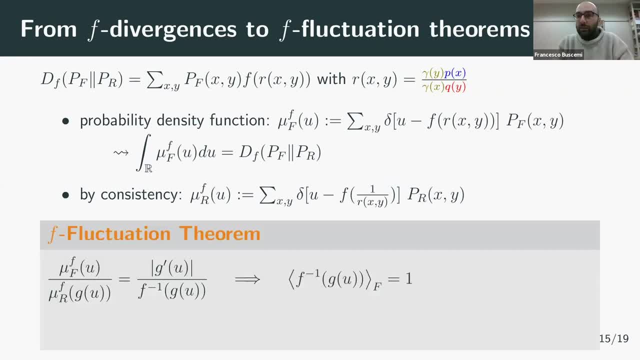 the reason I told you before, But still you can derive a generalization, essentially, of Crook's fluctuation theorem for various f divergences. So just you know, by just getting out of this physical, like this thermal narrative, just by looking at these things only, 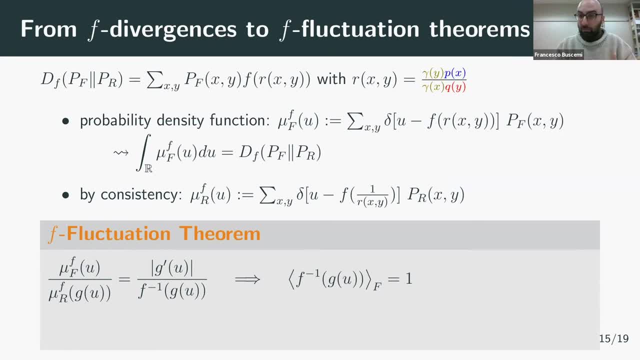 from the viewpoint of mathematical statistics, as just manipulating probability distributions. we have been encouraged to look at what happens for other divergences, Whereas instead, probably if we were just thinking about the thermodynamic interpretation of this relation, we would have been 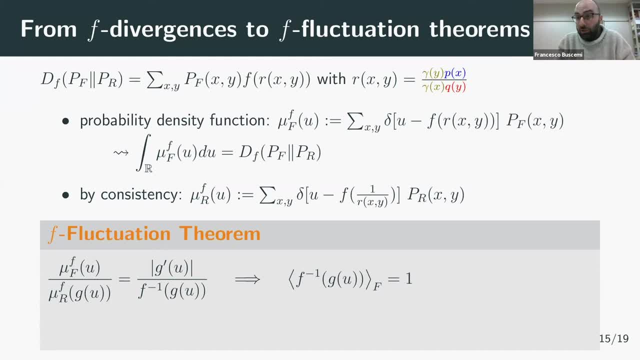 basically subconsciously bound to work with the logarithm, because the logarithm is the thing that gives you heat and work And all this kind right. But still you can have Crook's fluctuation theorem. for general functions It looks like this, And from here you can get an F? Yerzhinsky equality just by moving. 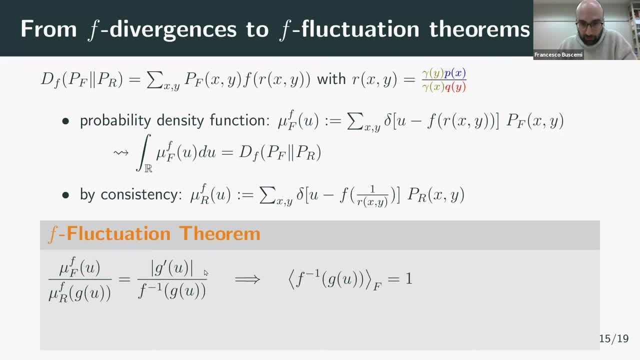 this reverse process here on the right-hand side, moving this denominator on the left-hand side, and then by integrating the right-hand side. it must be one, because you have exactly g of u and then you have the Jacobian. So basically they cancel out and you get one. Everything is. 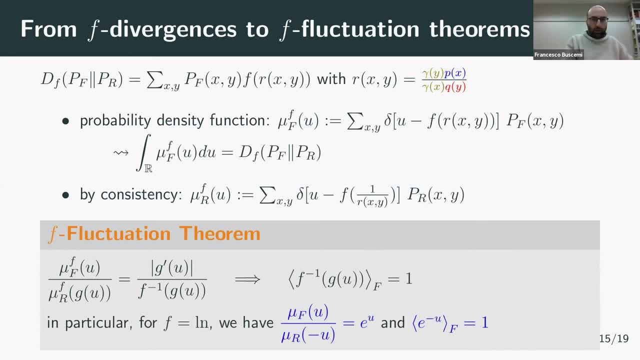 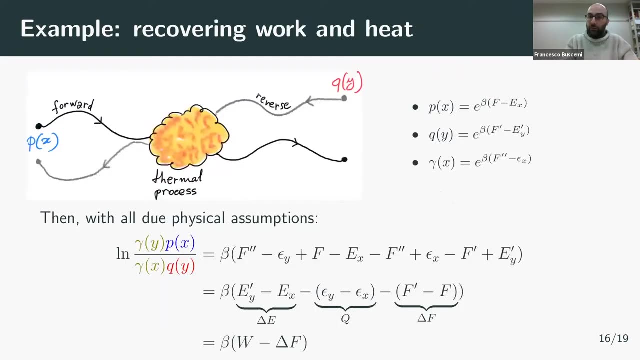 normal, As I said in particular, for example, if you choose F to be the logarithm, you reconstruct the form of Crook's and Yerzhinsky, But not only the form. This is something that I want to stress. 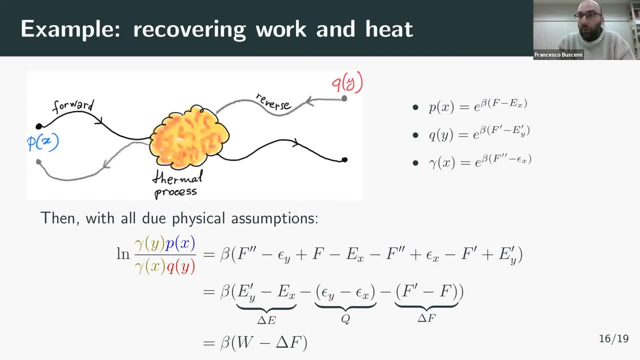 It is that, now that you have this general picture for fluctuation relations, now, at this point, you put the physics in. For example, you can recover work and heat without being bound to those assumptions of microscopic reversibility that, by the way, 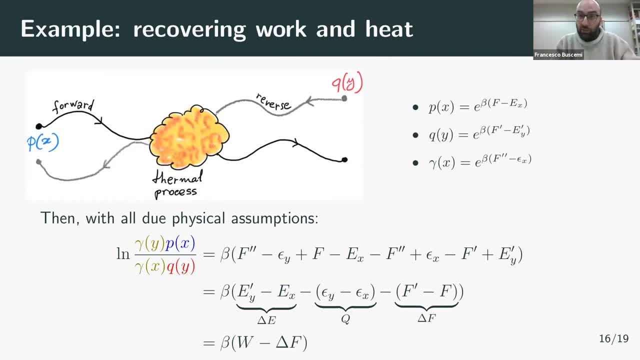 no one really knows the meaning of microscopic reversibility. Some people confuse it with detailed balance. There is a debate about it. What is the actual meaning of microscopic reversibility? But without referring to any assumption of microscopic reversibility, just by using Bayes-Laplace rule you can re-derive also the physics. 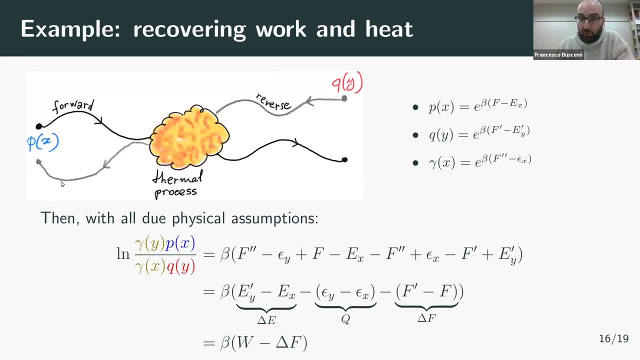 Once you do the right assumptions, of course. For example, you can imagine that now the initial distribution is a thermal distribution for some Hamiltonian. The final distribution, which is the initial for the retrodictor, the final distribution Qy, is thermal for another Hamiltonian. 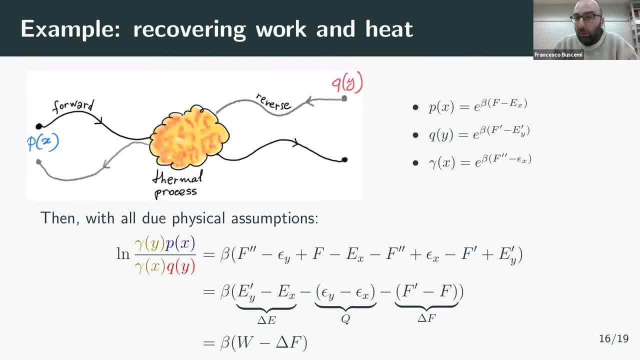 And now you can even put: you can just throw in for good measure some thermal process in between, So you can add some kind of stochastic evolution there, A thermal process that you can say that by definition any change in energy that occurs here should be accounted as heat. 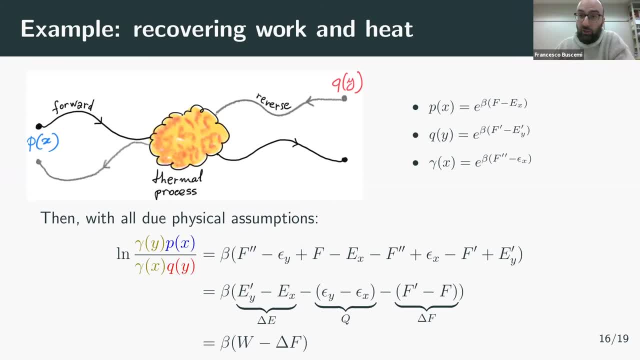 Because you define it to be a thermal process, like you might know, that it models an interaction with a bath or something. So with the right physical assumptions- and you can always find those if you want- but by looking at this ratio of probabilities you get exactly at the logarithm of this ratio. 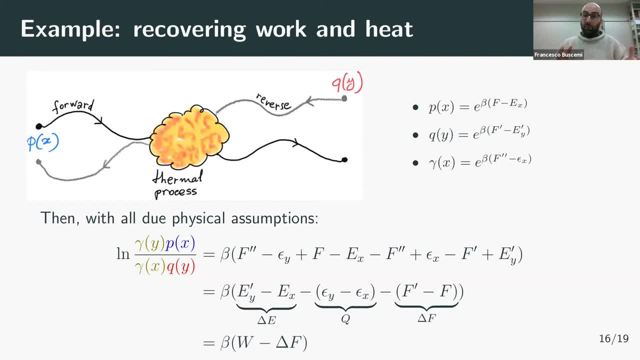 Which is the ratio that quantifies the asymmetry between prediction and retrodiction according to the Bayes rule, is exactly the thing that was there in Clausius' formulation of the second law, But this can be used in more general scenarios, And still we have to find a place where this simple, this naive, if you like, Bayesian approach to the construction of a reverse process doesn't work. 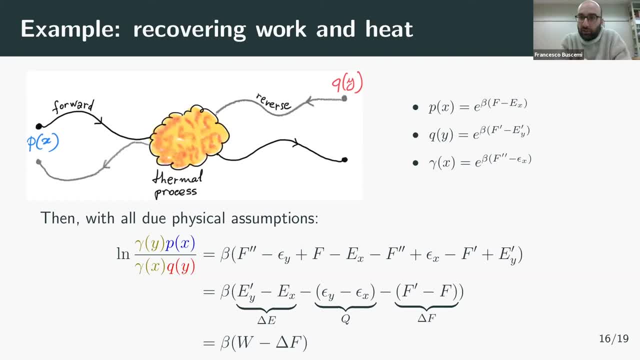 For example, we are able to re-derive non-equilibrium potentials, like those that appear in Hatano-Sasa-Ferrari's, that are a fluctuation of relations that are accounted for as an excess heat, something that is there but you don't know exactly if it seems something that you need in order to make equations work. 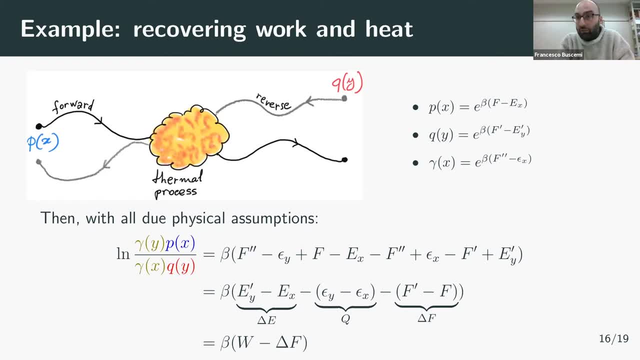 Well, you can just explain that as a remnant of Bayes' rule, And you can also look, for example, at the other stochastic process, for example, Langevin equations and so on. This is ongoing work, But we really believe that everything that you have to do is to apply Bayes' rule. 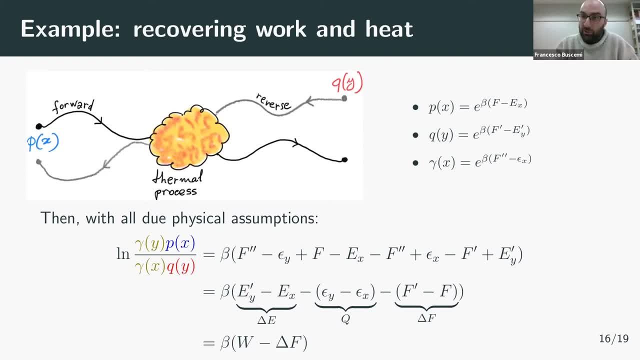 But we really believe that everything that you have to do is to apply Bayes' rule. So so fluctuation relations are essentially, they are direct consequences of not any macroscopic balancing mechanism, but just the correct application of Bayesian inference. And then you put the physics on top. 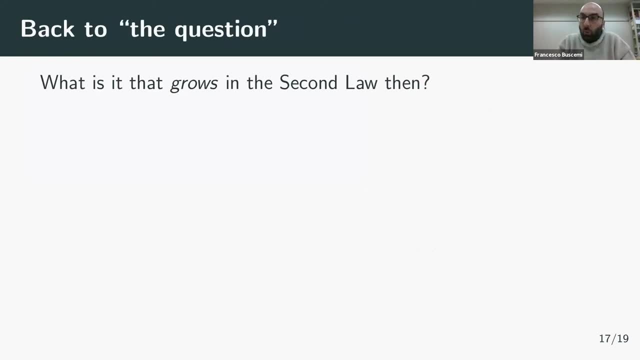 So? so back to the question. So what is the content of the second law then? What is that? what is it that grows monotonically in the second law? So, as Georginsky equality directly implies Krauss's inequality, 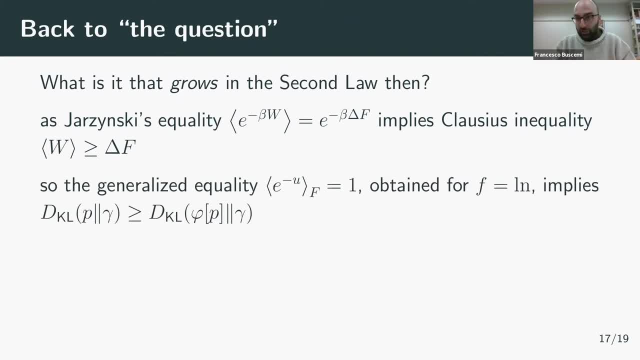 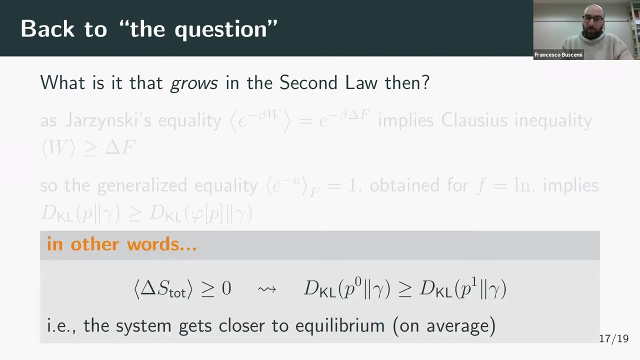 here you can take the generalized equality that we have for the logarithm and by applying the same equation, the same technique, which is just by using the complexity of exponential function, you reach this inequality. So, essentially, what is usually formulated as the entropy increasing in average in the formulation of the second law, 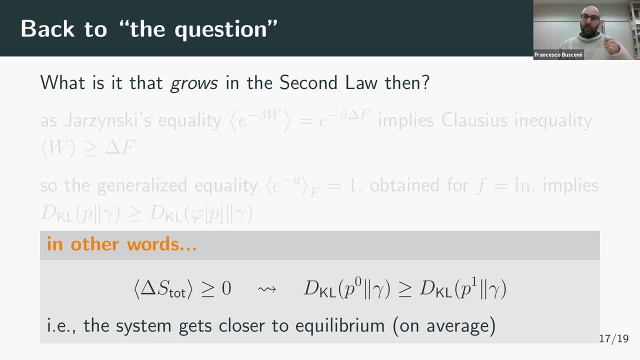 can be more generally understood as the idea that the system gets closer to equilibrium on average. because, you see, this is the divergence, the relative end entropy between the state of the system and time t0 and the equilibrium distribution. In a sense, 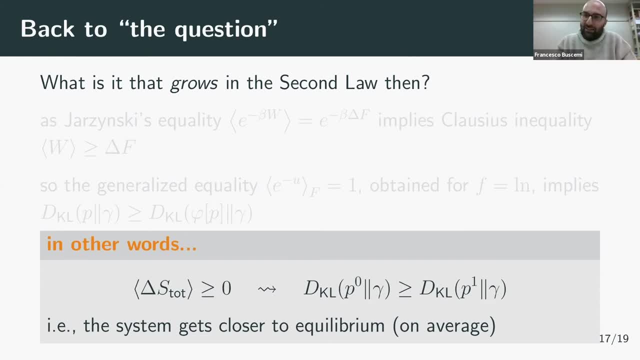 the second law again. if you get stuck in some fancy party by someone asking you the content of the second law, don't run away but just say it's easy. it tells you about the fact that these one wayness that we perceive these extreme and balance between prediction and retorde. 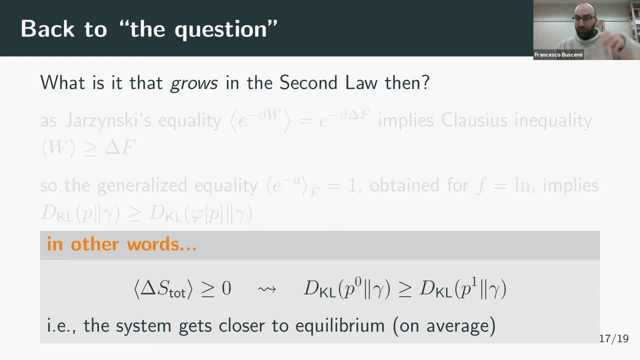 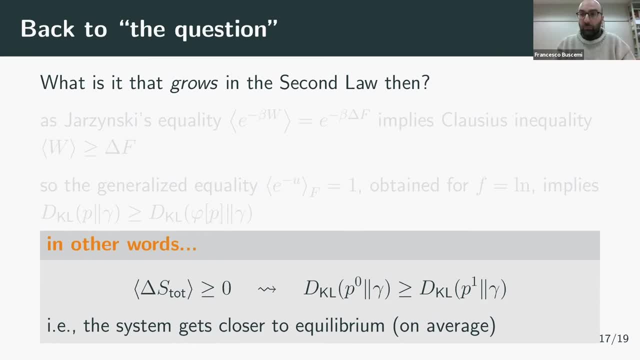 prediction in time and retrodiction in time: uh, goes down, this one-wayness goes down. so essentially well, this can be understood as saying that any situation out of equilibrium gets closer and closer and closer to equilibrium, condition where this one-wayness is: uh, not there. 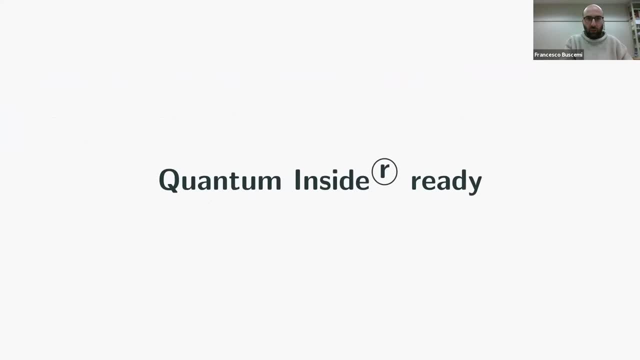 anymore. um, so, and now my um final remark about. i mean, this was a. this is the symposium of the center for quantum mechanics, quantum technology. so where is the quantum in this talk? so the thing is that, well, our motivations were starting from trying to understand fluctuation relations in the quantum case. 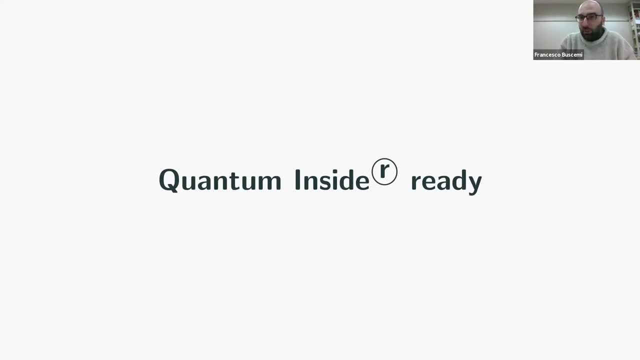 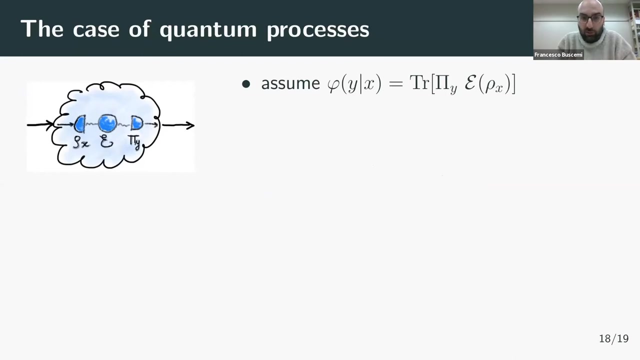 um, but now in this talk this look as a kind of afterthought, but the point is that this approach, by using a sim, the asymmetry between prediction and retrodiction is quantum ready, quantum inside ready. you can just plug quantum boxes inside this stochastic process. so you can imagine. 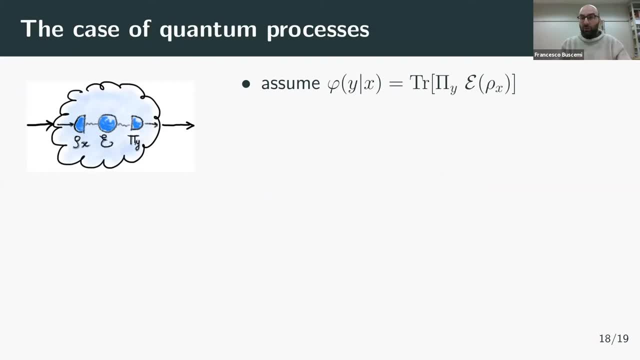 that this stochastic process between x and y is actually caused by some quantum mechanism where you have some states, rho x, some evolution, cptp channel, completely positive charge preserving channel, and then some measurement with some pov and py and you reconstruct, you go back to what i told you before, just by using the formalism. 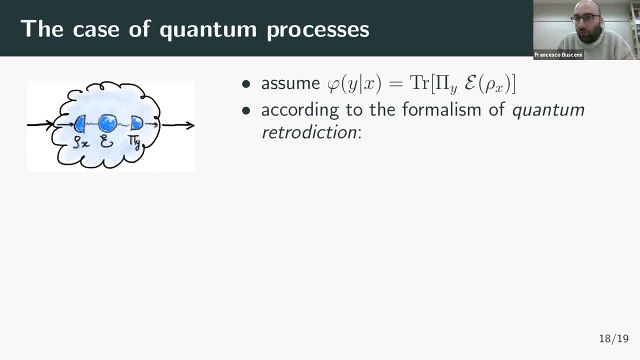 of quantum retrodiction, which is something that is there in quantum theory, it's not extremely popular, uh, basically because- probably because, as ruth said before, it is kind of the young of uh, quantum theory- people prefer to predict and retrodict, especially because prediction gives you an idea of controllability, like you prepare initial conditions and then you see them evolve. 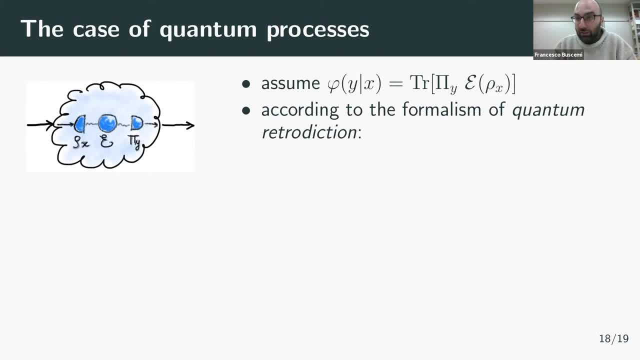 in time. but sometimes you you're not allowed to do that. actually, one could even argue that even in quantum theory you never really have the chance to really figure out what's going on in quantum theory. you never really have the chance to really figure out what's going on in quantum theory. 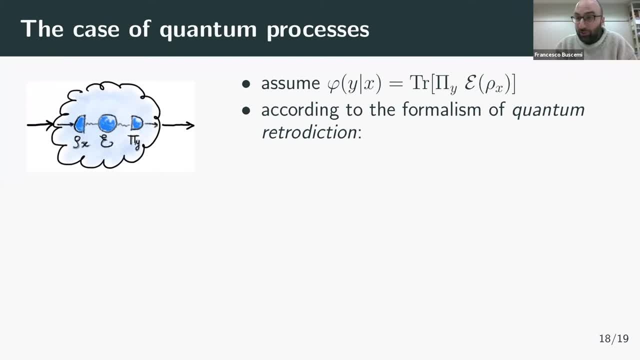 you never really have the chance to really figure out what's going on in quantum theory. you can just prepare some experiments that you hope produce correlations that are explained by the theory. but that would bring me to another direction. so let me just continue from this point. so just by applying the formalism of pattern retrodiction, which is as follows. so you take the 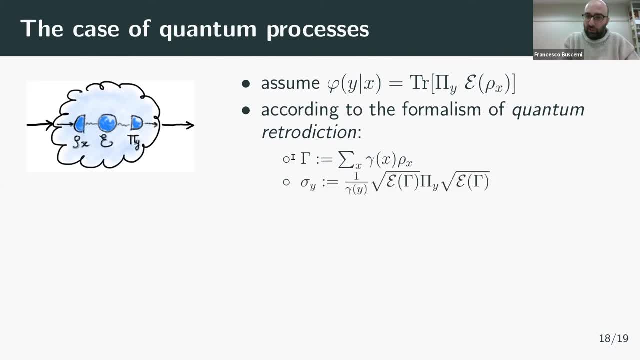 distribution that is invariant for the process, and you construct this average state gamma, which enters into the construction of some density matrices, sigma y, that are constructed from the povm element. analogously, from these states, rho x, you are able to construct now povm. so what were states before? 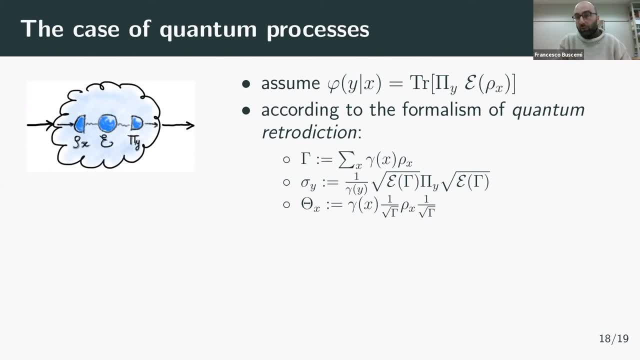 become povm for the retrodictor, and what were the povm for the predictor become states, the things to be plugged in the process by the predictor. and then the channel becomes this thing, which is the pet's reverse channel that is ubiquitous in quantum information theory. 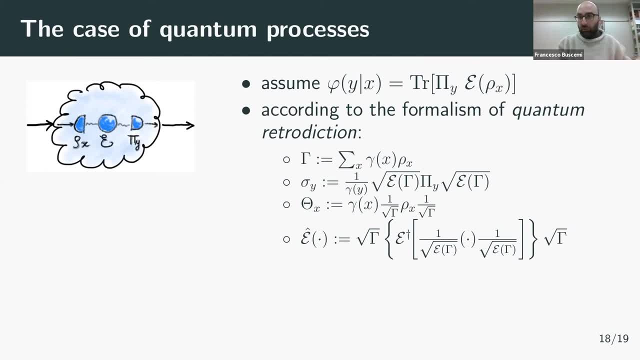 so pet's reverse channel can be seen as the quantum retrodicting channel, the quantum reverse process, the quantum jeffrey's rule. all these things coincide. the quantum jeffrey's rule is pet's reverse map and by using these three objects you can actually 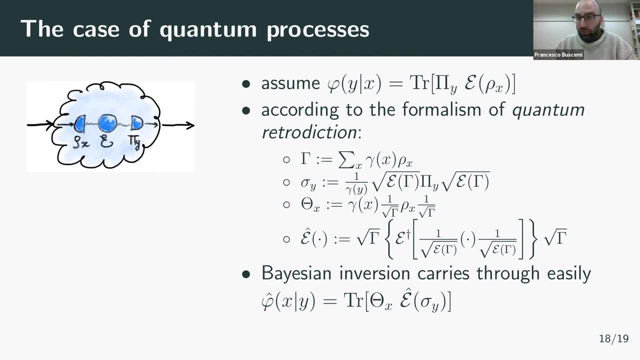 construct a physical reverse process. that is exactly what beyer's rule would tell you to use as the reverse channel this phi hat. so this is the picture. so you see, we just flipped the arrows of this box inside out, and what was a state now is a povm. what was a povm is now a state, and what was a. 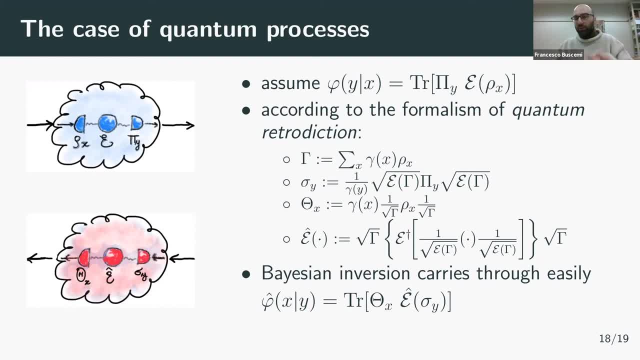 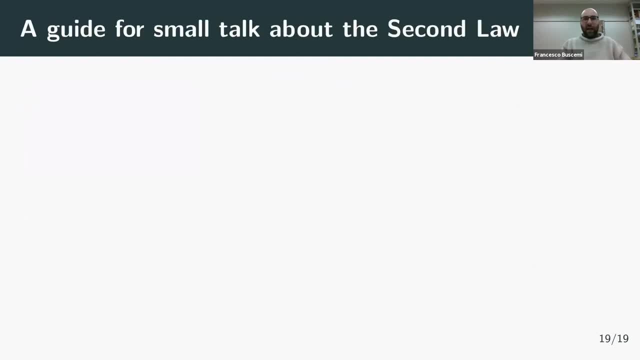 cptp map is again a cptp map, but flip around, it is the reverse pet's channel. so conclusions: so a guide for small talk about the second law. so when the entropy always increases, stroke doesn't help. you can try with these, one of these or any of these at your choice. so out of equilibrium there is a symmetry between forward. 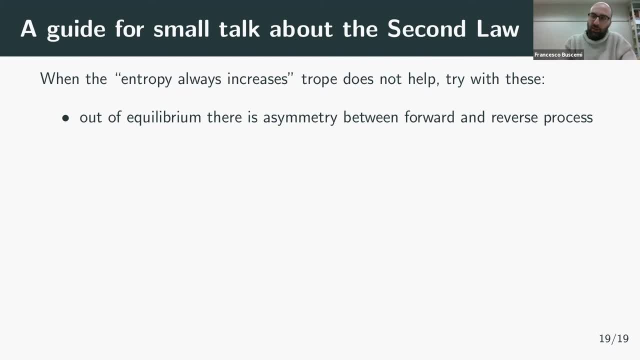 and reverse processes and we understand this as an asymmetry between uh predictive inference and retrodictive inference, and such asymmetries, astronomically conspicuous in macroscopic situations- and this is our perceived- could be understood as our perceived one-wayness time. by the way, there's a beautiful talk by richard feinman on youtube about past and future, where he 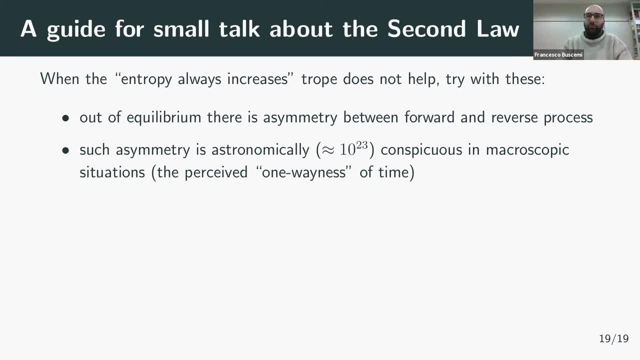 basically deals with this, this topics- and again, feinman was there in the, uh, retarded waves that ruth mentioned before. so, and then we, we, we also see that such a symmetry is well described in terms of fluctuation relations. but the point that i want to stress is that this fluctuation relations should be seen, or can be seen, at least, not as consequences. 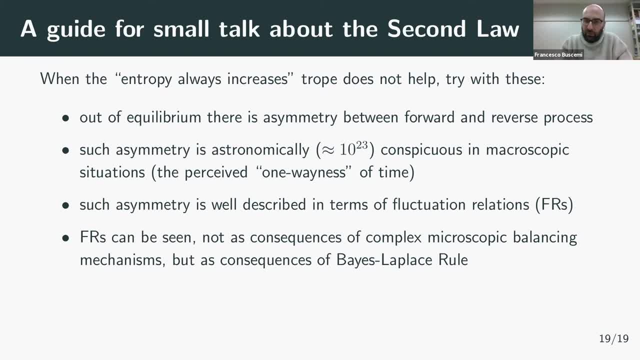 of some complex, microscopic balancing mechanisms, but as consequences of just basel plus rule on its own. so, basically, consequences of consistent logical thinking. if you are a consistent agent, if you are a rational agent, you, um, you will notice this asymmetry between your predictive power and your retrodictive power, and such a symmetry is what is a 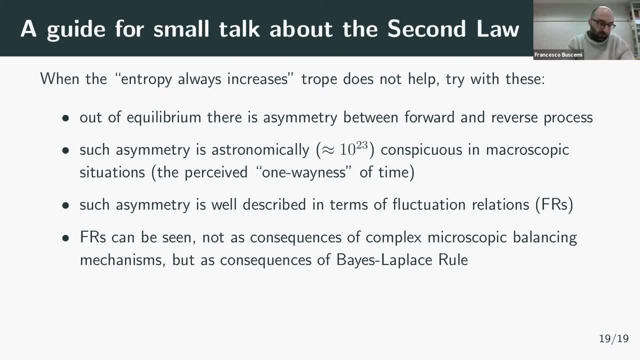 what lies at the basis of fluctuation theorem. hence fluctuation relations and the second law hold without physics. so the data processing theorem in information theory is exactly a second law without physics. there are no hamiltonians there, there is just information being propagated. but still the data processing theorem is a second law. uh, for information theory. 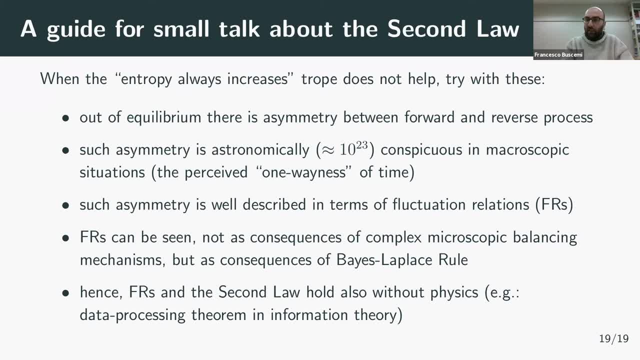 and on this i i stop and i thank you for your attention. okay, uh, thank you, francesco, for your talk. uh, well, i don't have any question in the uh, in the chat, uh, so, uh, i don't know if anybody wants to ask a question, or um, there is, i will ask. yes, howard, please. 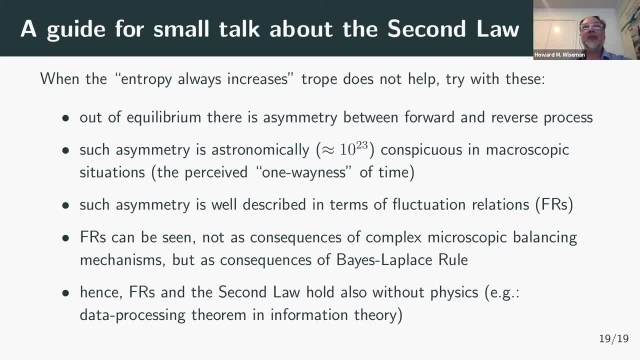 uh hi, francesco, hi, uh, thanks for thanks for the nice talk. um, so it, this is probably a very, uh, very basic conceptual question. um, but you, but your answer to your simplest answer to what is the second law about, uh, was: the system gets closer to equilibrium on average. yeah, yes, um, but so we? 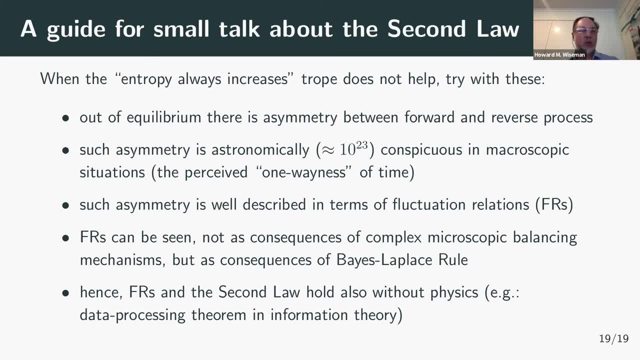 are. when we are talking about equilibrium and systems, you're talking about a probability of a probability distribution, uh, and. but then you have also have the on average, which suggests that there's an extra level of probability now in the, in the original, if i understand correctly, in the. 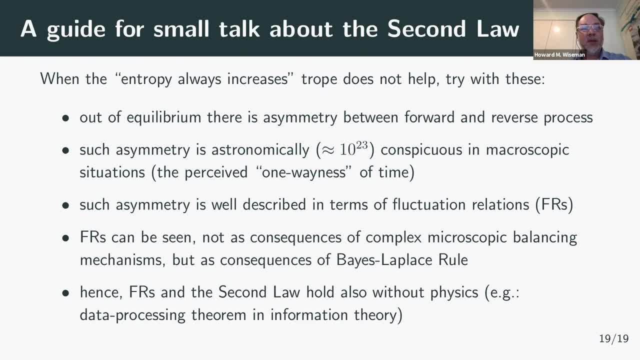 fluctuation theorem that extra level is the is is determined by the work done and that that work done is something which you actually know but which is stochastic. am i understanding correctly? yes, yes, i think so, yes, okay, so so then, if you said: uh on, but but actually the theorem that you 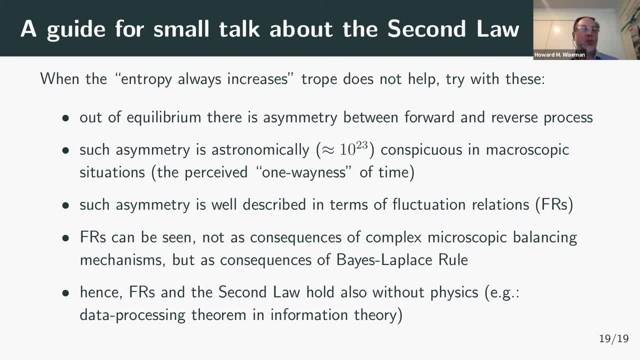 have this, this infinite class of theorems, which is more general than talking about work or whatever. then how do i understand this, this extra level of stochasticity, what, what? what does the on average mean when? why do you? yeah, do you need to include it in saying that the system gets closer to equilibrium on average? so, um, 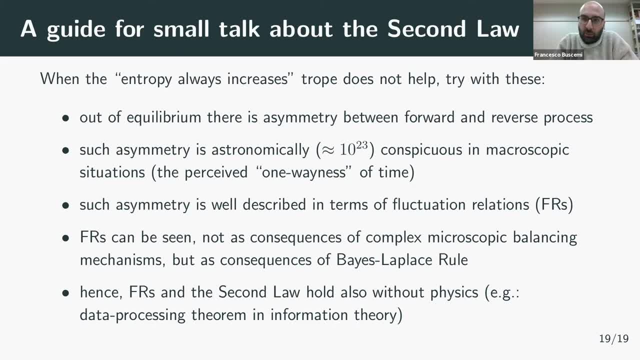 um, so let's say that there is a system which has some states and the states are are given according to some probability, right, and then there are probabilities on trajectories, so probabilities for which your state can go from state x to state y. so these are exactly the same that you get in the usual. 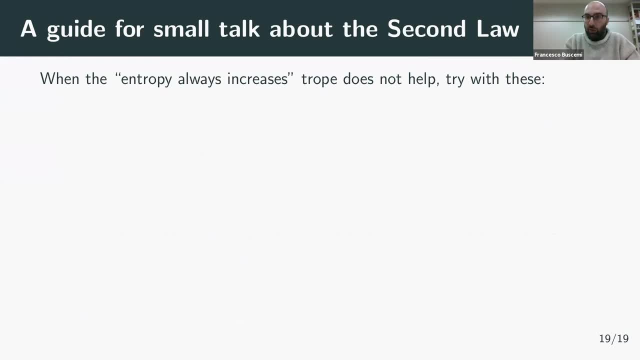 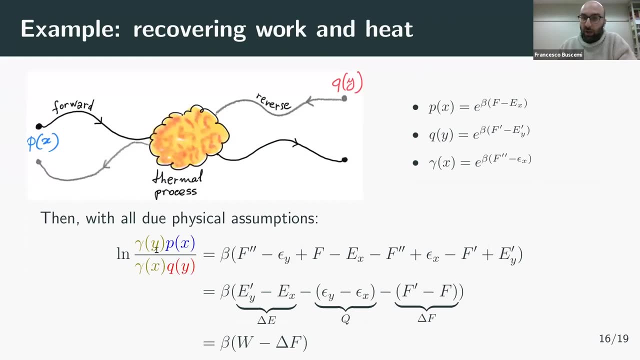 in the usual work, the usual work heat formulation of, as you can see here, essentially this ratio here is exactly the thing that gets averaged and becomes the random variable whose average essentially measures this asymmetry right. So I'm not sure if we are talking about exactly the same things When you say that there are two levels of. 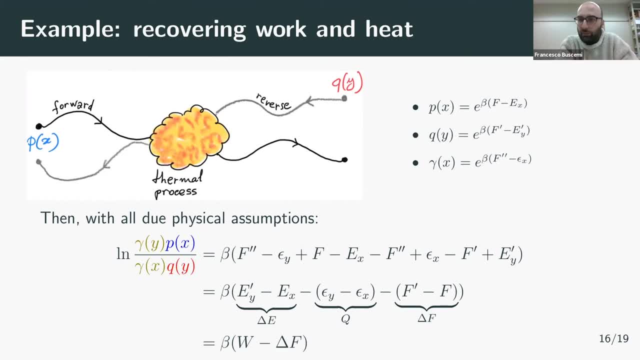 averaging. I don't see here two levels of averaging. Here you have a joint distribution on x and y. Basically this defines the process. Then one could think- I agree with you- one could think about a distribution over distributions, if you like, When you do this kind of Bayesian. 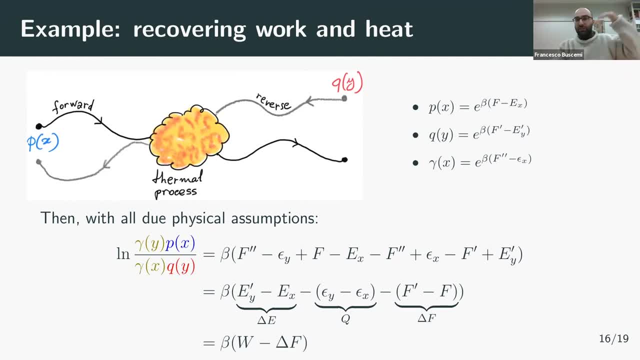 statistics you can always imagine hierarchies of Bayesian levels in which you do your inference. right Here we are at the most basic one. So here we haven't introduced any further level of average. So I'm not sure. Does it have? I don't know, I don't know, I guess, I still, I'm not sure. 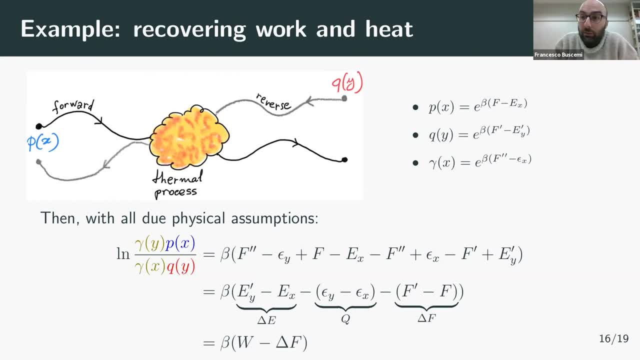 I still don't quite understand why you need to, yeah, why you can't just say: the system gets closer to equilibrium. Why is that wrong? No, no, that's correct. The system gets closer to equilibrium where, at equilibrium, you don't have this one-wayness of inference. 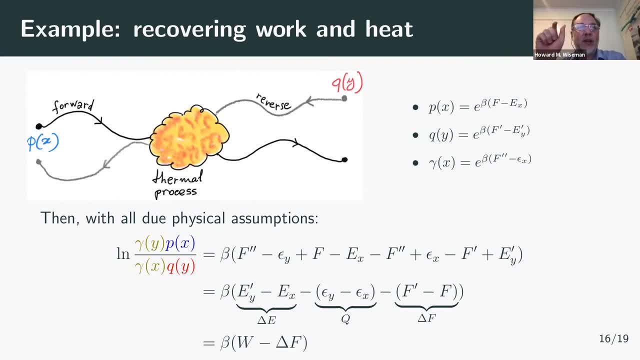 But then you said that, but then you explicitly included the on average caveat to that when you said that that was the correct Oh, oh, you mean, you mean that kind of initial initial thing. Well, it was. it was towards the end of your talk, I think. I mean. 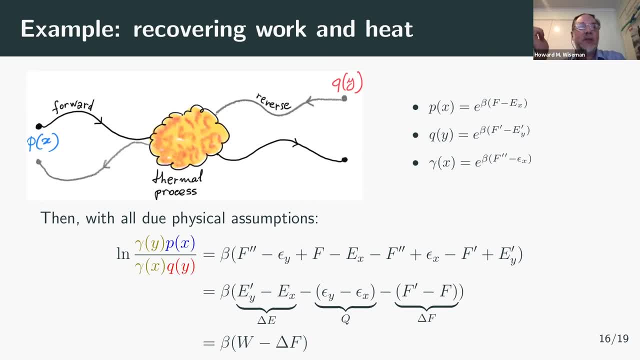 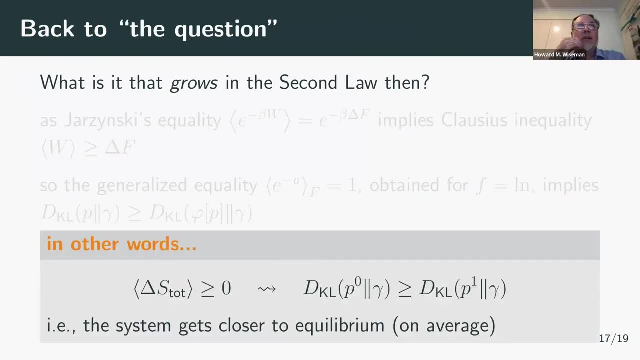 when you came back to saying: what is the second law about? Yes, Well, because, okay, oh, this on average in parenthesis here: Yes, Okay, Because you can see, basically that this, what is a relative entropy? Relative entropy is some. 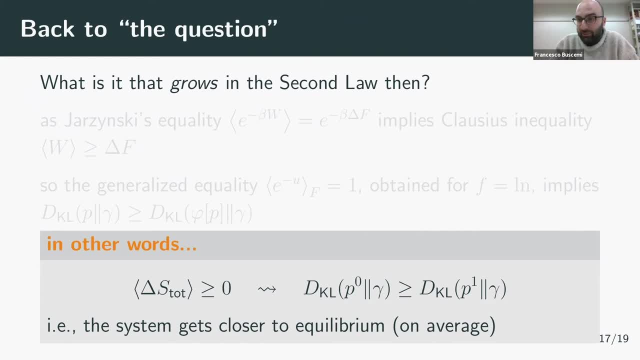 average surprisal Right which suggests that it's So. so a relative entropy by itself is something that we use as a distance measure, but relative entropy is in in itself. is the average of something? is the average of this random variable? Yes, That is constructed starting from the ratio. 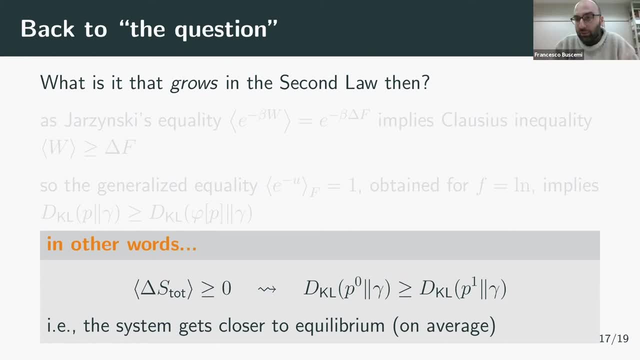 of the two probability distributions, Then we tend to forget about this fact. but it is something that tells you about average things. right, It could be that for some realization of your experiment, you would see that maybe just just by looking at information theory. Okay, Let's, let's go abstract, Let's forget about about work and heat and so on. 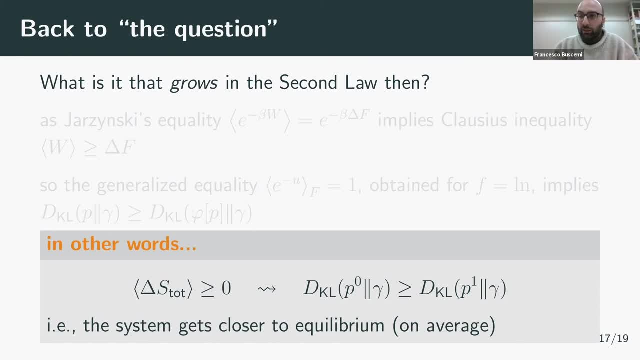 But it could be that it's some realization. it seems that the the information goes up. Maybe you know Bob is able to guess exactly what Alice put in a in a in a noisy channel- And then it seems that in this realization there was a kind of increase of of you know some, you know some, you know more information. 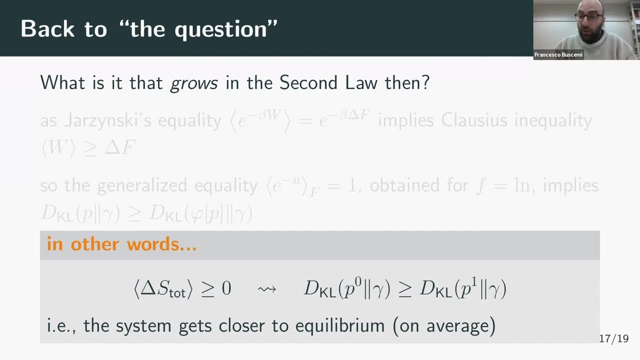 And then you multiply that by the number of other variables, so you can see that. So that's pretty much a� of information, because Bob was just lucky in that occasion, Because the data processing inequality tells you that the distinguishing point- But in that sense isn't the system- 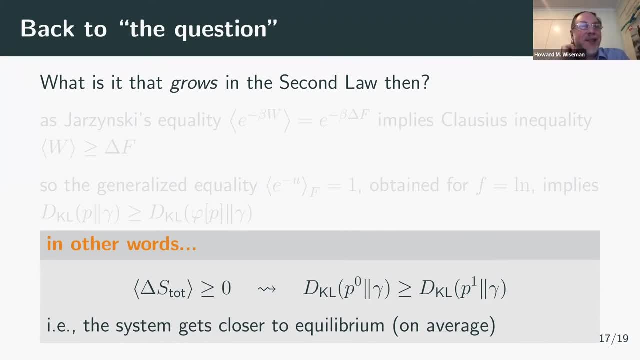 out of equilibrium in every individual run, then I mean, the notion of getting closer to equilibrium only makes sense in an average sense. Is that true? Yes, I would say so. yes, Right, OK, OK, OK, I think that answers my question. 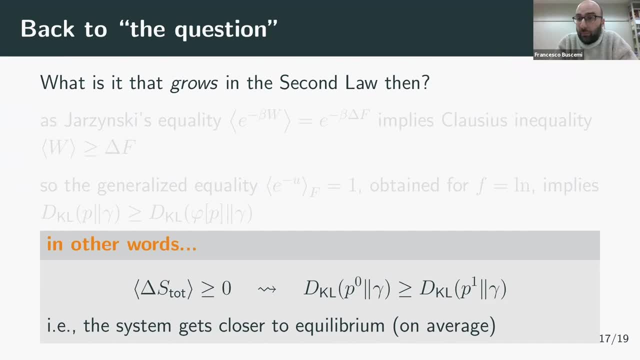 And microscopically, the average is all we see, Always what. And microscopically, this average is all we see, basically because these distributions become extremely piqued about the average value. So, for example, in a thermodynamic experiment, 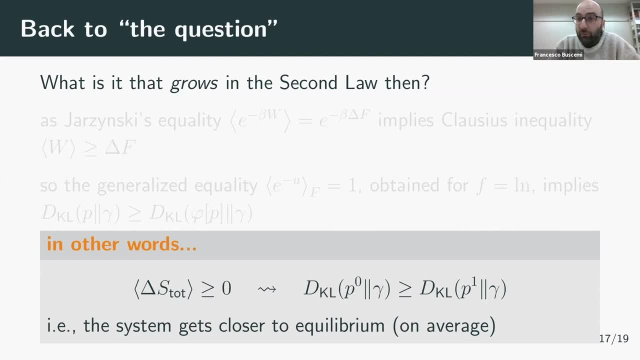 you can say that work has some definite value, But when you have a Very small system, then work will actually fluctuate. You can repeat the same thermodynamic protocol many times And each time you will find a different value for work. 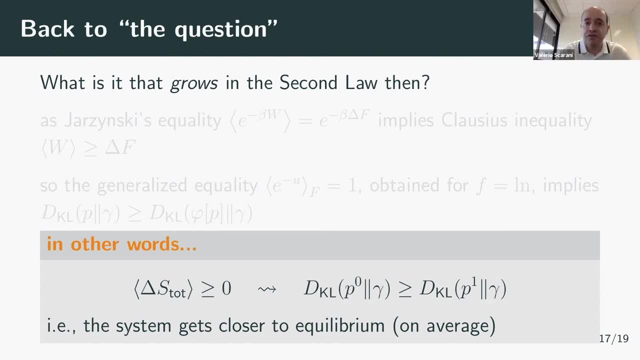 OK, may we move to another question. There is a question by Miele Gu. If Miele wants to unmute himself and ask the question- And I think unfortunately it will be the last question because we don't have time And I'm sorry for whoever else wrote some questions here- 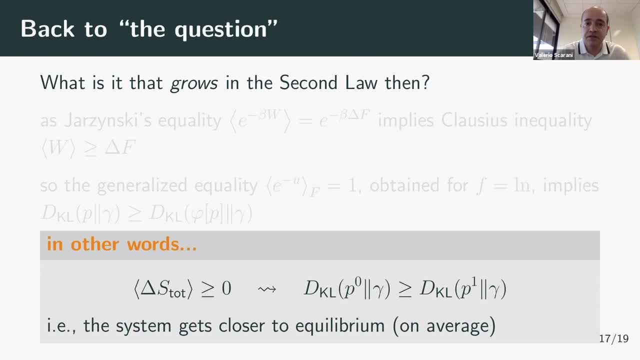 But Please, Miele. OK, great Thanks for the nice talk, Francisco. I guess I'm very interested in your perspective here that the second law of thermodynamics is essentially an information Bayesian concept, It's origins, And I guess this is one of those hotly debated topics. 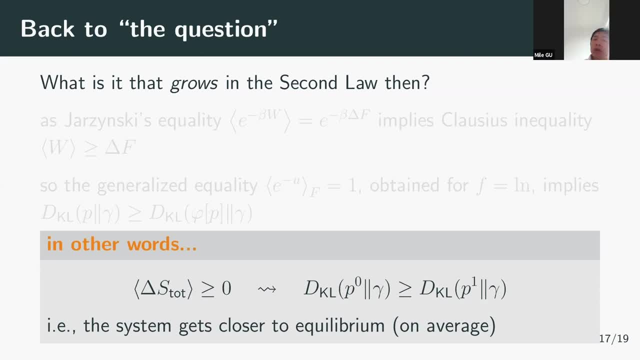 But in your opinion- I want to see what you think of- Is the framework that you are proposing, the basic idea that it's our state of knowledge of the system that tends towards the equilibrium? Because, from my understanding here, everything here applies regardless of whether the universe is unitary or non-unitary. 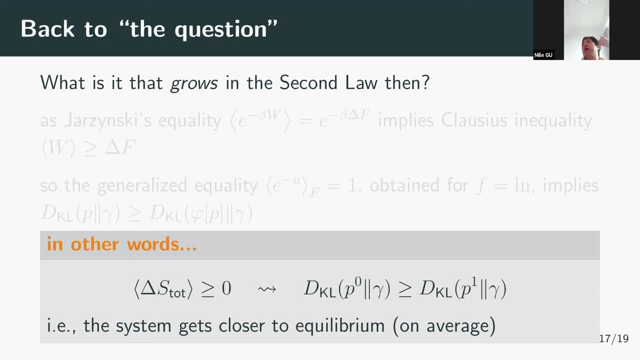 And it's really just about our measurement statistics at time a versus time b, And the asymmetry of prediction and retrodiction caused by- well, the asymmetry from the Bayes theorem when applied to thermal equilibrium distribution. So, as you demonstrated, there was very little physics. 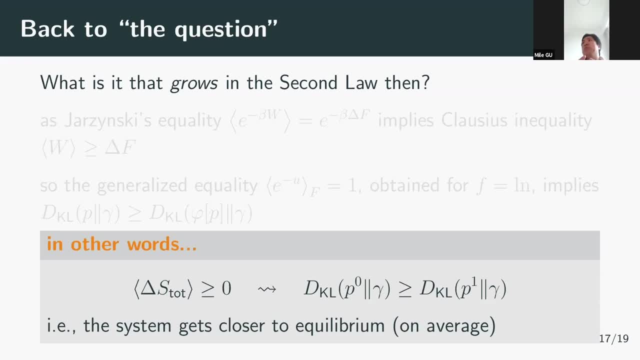 in that entire argument. So can we say that this second law of thermodynamics- in your opinion one of the origins or the origin- is really a statistical law where our expectations tend towards some sort of equilibrium, assuming that equilibrium happens to be the Gibbs distribution? 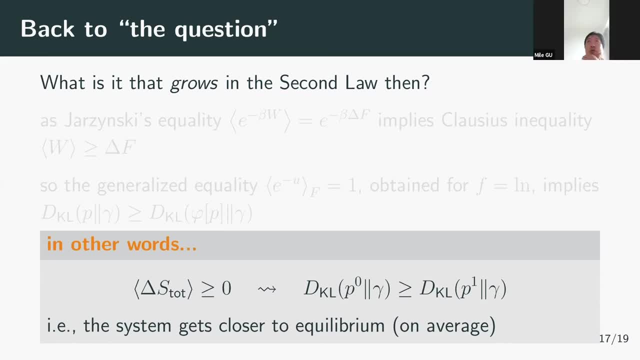 Well, equilibrium need not be the Gibbs distribution necessarily. This is the first thing that I would like to stress here. And then, if you want me, if you want to bring me on the fields of what is the interpretation of this prior? basically, 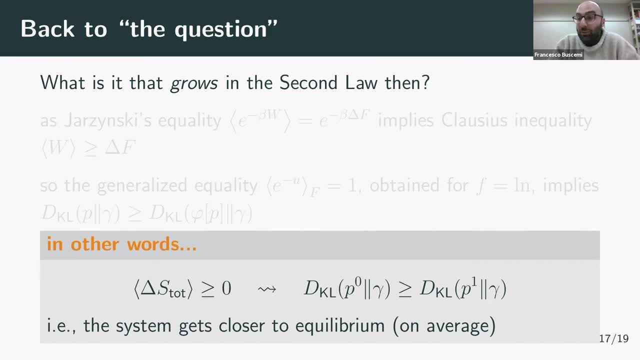 what is the probability, whether it is subjective knowledge or whether it is objective knowledge, then I'm not going to follow you here, I don't know Like. I'm just saying that you can derive these theorems that were at least by looking at the literature around. 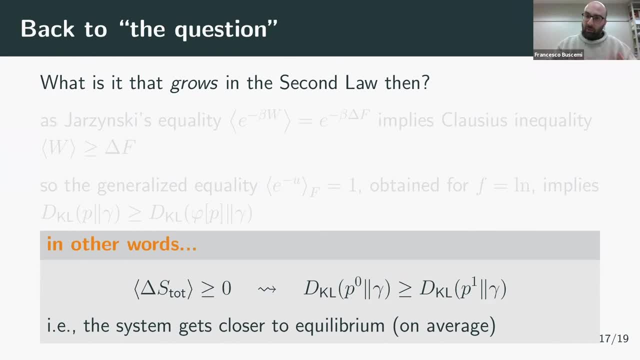 were always looked upon as something emerging from some stuff doing stuff at the bottom, some Hamiltonians and system interacting in such ways to preserve this microscopic balance of things baked in the bottom. You need not that, So you need not have any model of interaction. 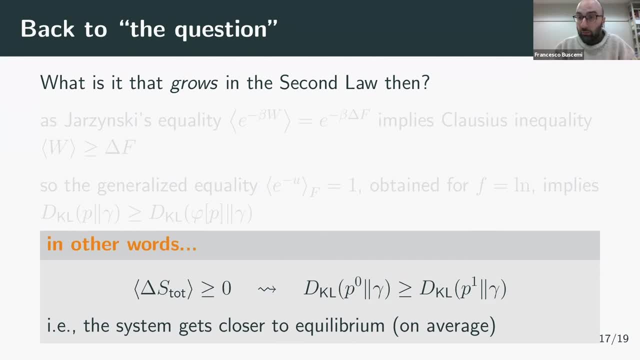 before saying whether a fluctuation theorem holds or not. This is a truism that comes from Bayes-Laplace rule. So basically, you can derive fluctuation relations all the time, everywhere, like for things that have nothing to do with physics. 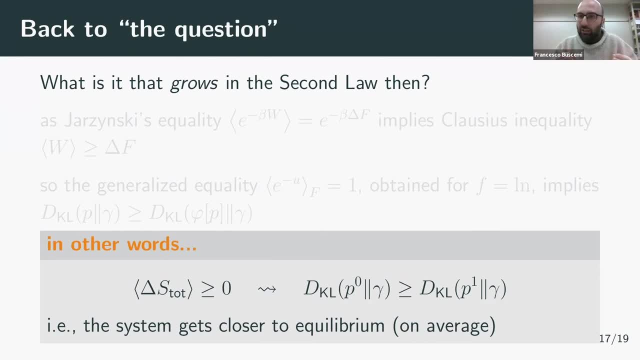 You do not need any balancing mechanism. That's the point. I want to reject this idea of mechanism that is at the bottom of fluctuation relations. So then, Kai, I have a question. I have a quick follow-up on this. So my understanding with thermodynamics: 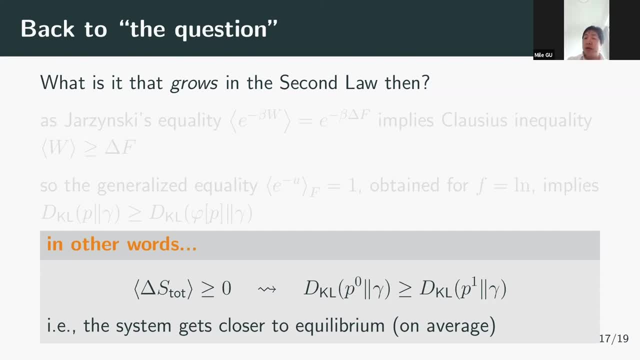 is that the macroscopic variable in temperature, that once we have that fixed, the maximally entropic object that we have is a thermal state. So it kind of makes sense for that to be as a prior. But would you expect a whole range of different second laws. 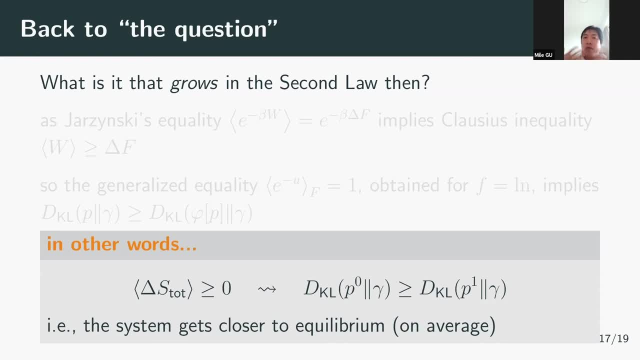 for other systems where a reasonable prior is a completely different distribution. So in a sense, can we generalize the second law to not just say a non-thermal equilibrium distributions using this sort of framework? KAI LIPINDALE- Well, here actually, 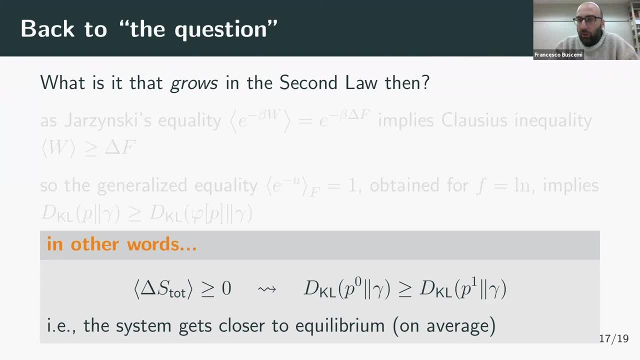 I started constructing the reverse process from equilibrium because fluctuations are usually considered around equilibrium, But Bayes-Laplace rule does not need that. You can construct the inverse probability from any initial condition, even though this initial condition is not at equilibrium for your process. 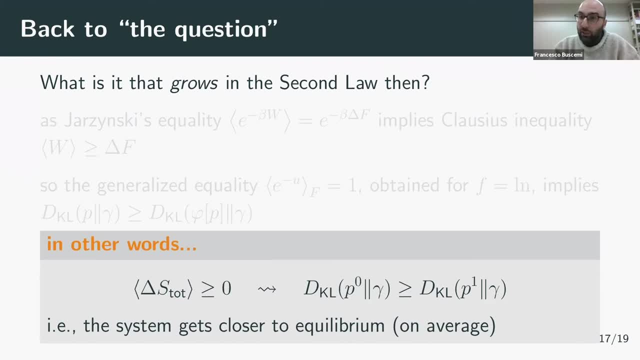 So, in a sense, you can actually write things that look like fluctuation relations, that tell you a relation between prediction and retrodiction, even out of equilibrium. That's super interesting. So that's something you're exploring at the moment. KAI LIPINDALE- Yes, 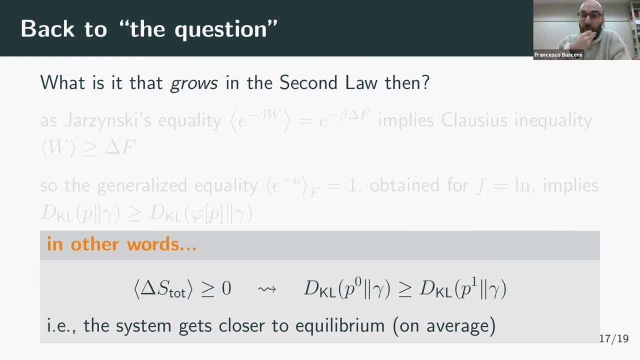 Like we have a program with Valerio to try to see how far we can push this intuition, But I'm pretty optimistic that actually this is a good way to think about this. This is really interesting. Thanks for that. I'll have to catch up with Valerio as well. 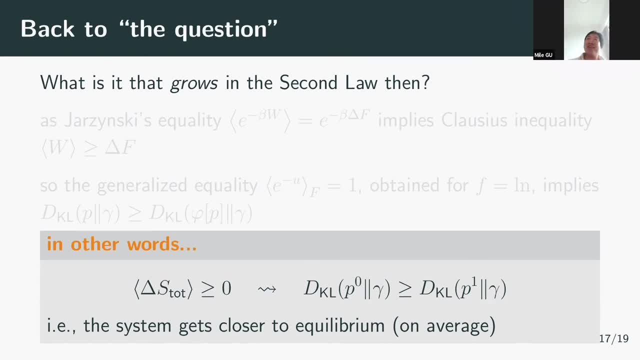 about this at some stage soon. OK, great Thanks for the talk. Bye KAI LIPINDALE- Excellent. Bye, Francesco. I have to tell you that we received quite a few other questions that I tried to answer myself.